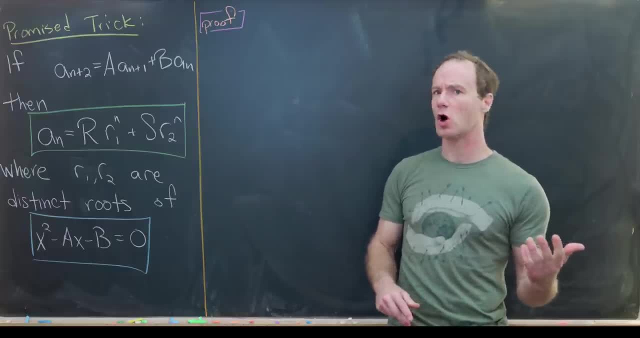 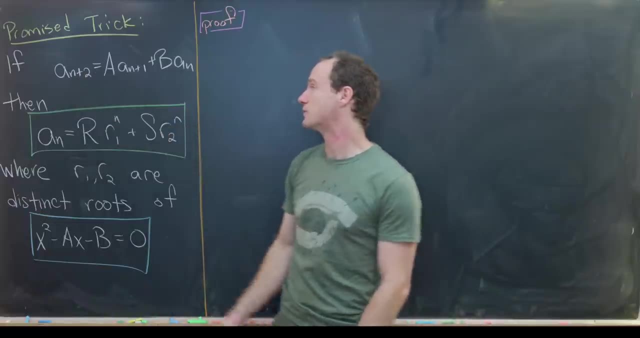 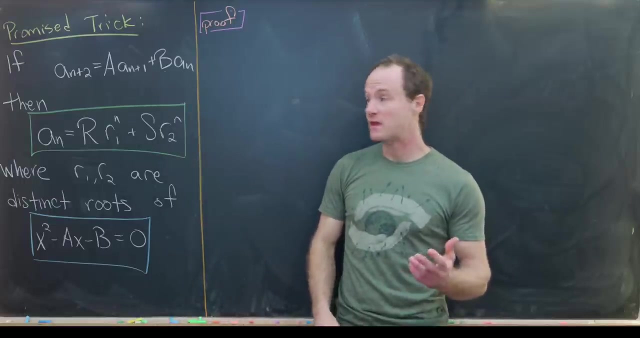 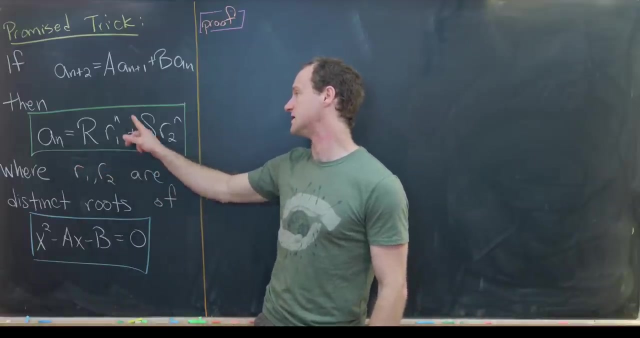 where we go over that trick. Okay, so let's recall what we did back then. So if we've got this recursively defined sequence a? n plus 2 equals capital A a sub n plus 1 plus capital B a sub n, then we know the closed form for this sequence. a? n is of the form capital R, r1 to the n. 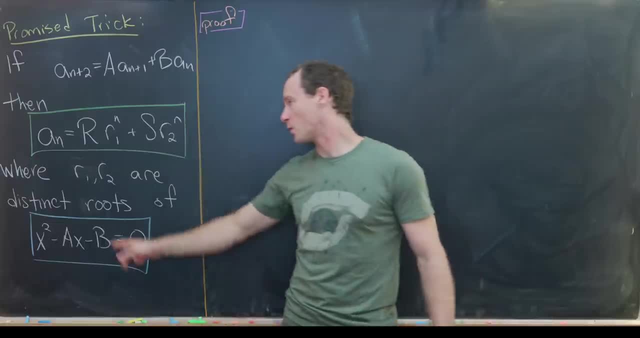 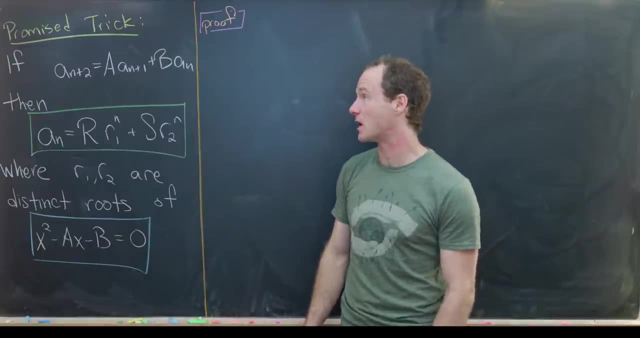 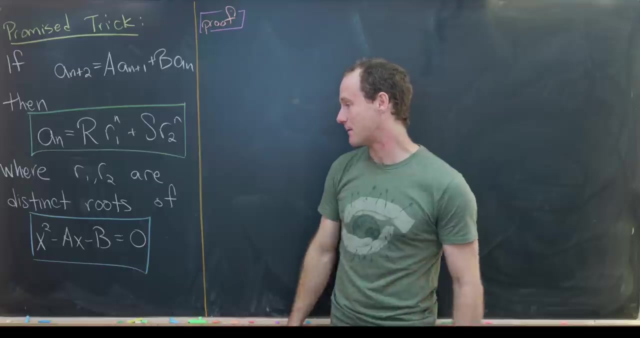 plus capital S, r2 to the n, where r1 and r2 are the distinct roots of the following polynomial, which is known as the characteristic polynomial Related to this recursive sequence. So we've got x, squared equals ax, minus b equals 0.. And you 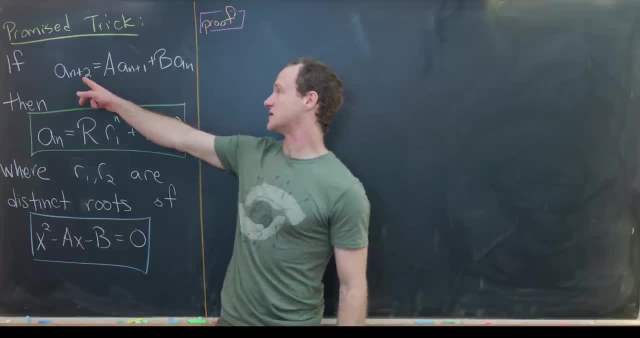 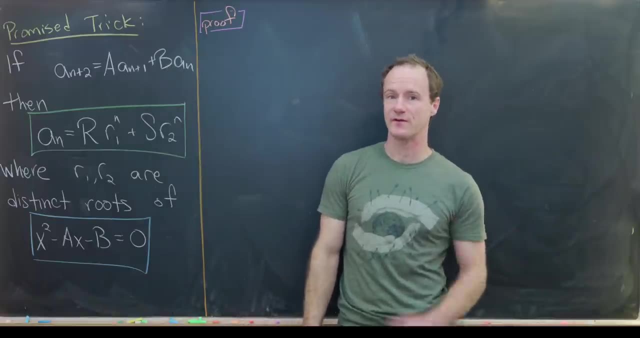 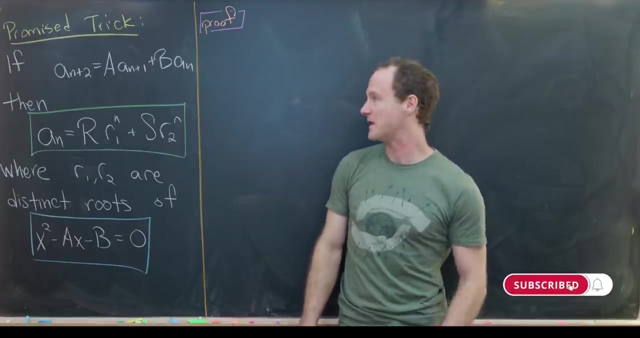 might say: well, what about the seeds? And so this allows us to define the n plus second term in terms of the n plus first term and the nth term. Well, what about the zeroth term in the first term or the first term in the second term, depending on how we define this? Well, it turns out that 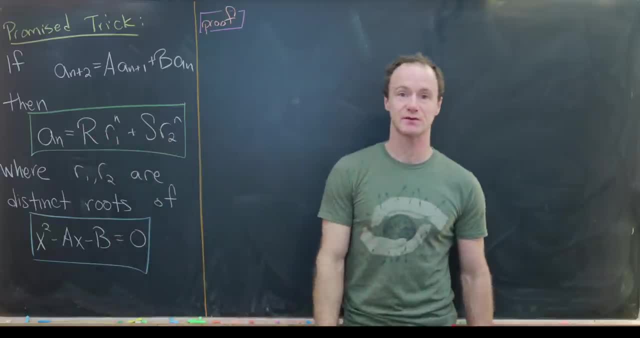 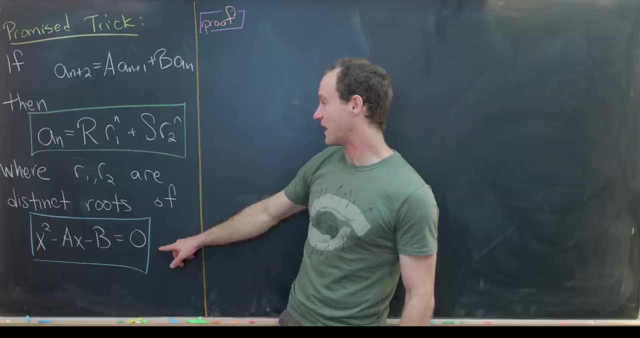 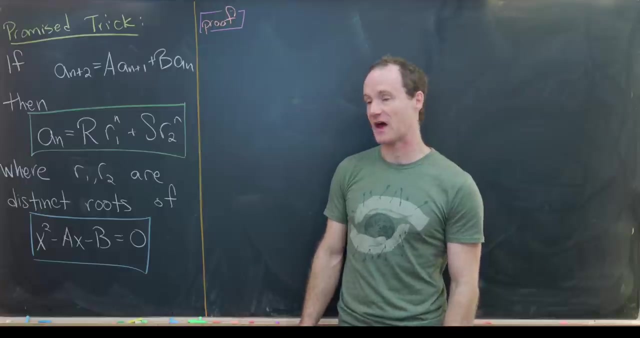 we use the function tilde. So there you are. whatever we're how finding the roots. So I think many people will be forced to figure this out, but I do want to add this out because, again, it's important that we do look at absolute negative employment accents. So that's always something you would. 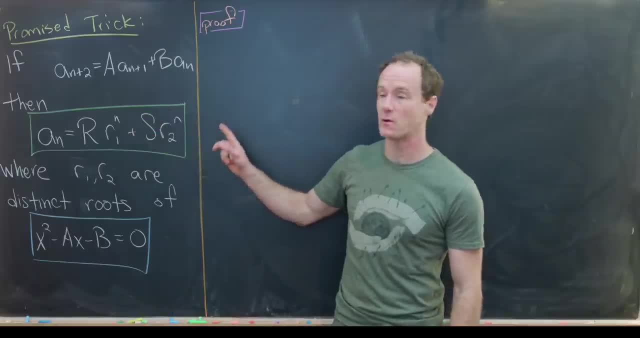 consider when employing this if you have any snapshot. So I just added a little vois and now we can go back to the reverse. I don't like that. But yeah, do have to go back and is: does that? do all the work, Do all the confusion from the beginning? and some of you Here it is, This is a perfect, that kind of 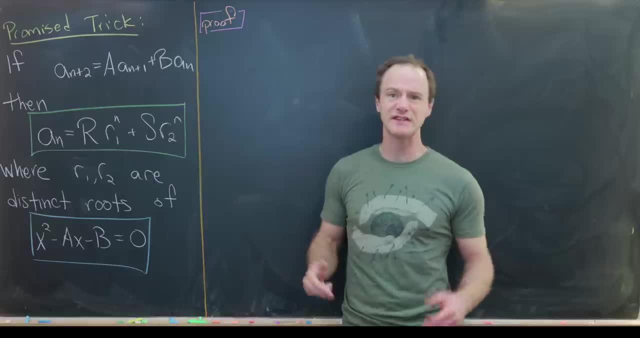 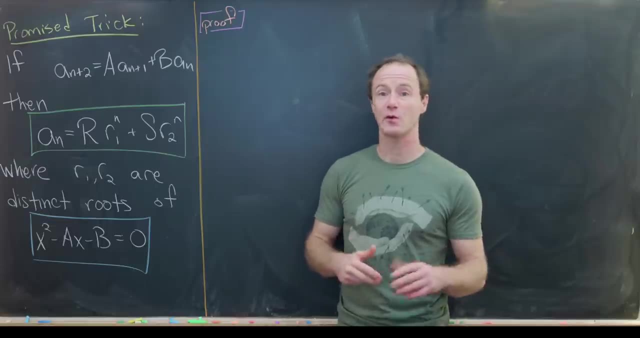 it. Well, sure, what is the standard proof of the closed form wheels? Yes, this favoriteーホ, this recursion, And that's a reasonable way to do this, because obeying this recursion has some sort of uniqueness property. But that's not the way we're going to prove this, And that's because 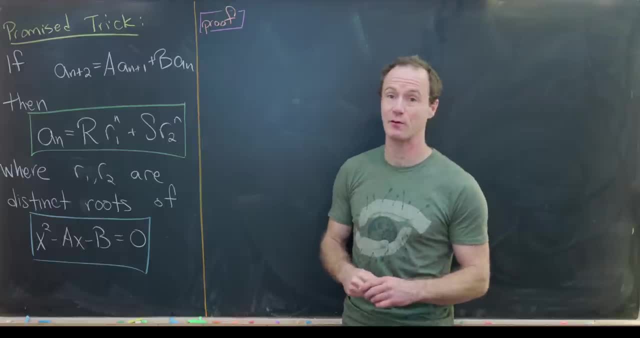 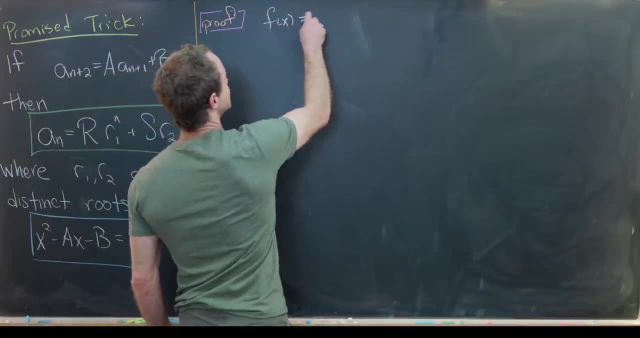 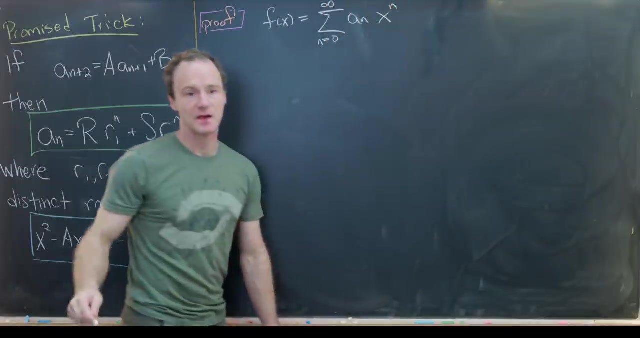 to a fault. I like to do things constructively And that's exactly what we're going to do here. We're going to use a generating function, Okay. so let's start off by defining f of x to be the sum- as n goes from 0 up to infinity- of a sub n, x to the n. So, in other words, that's our generating 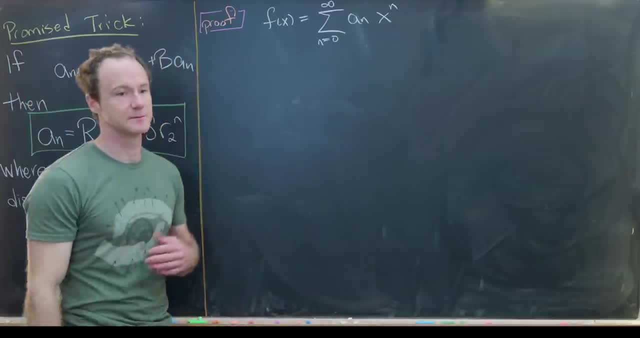 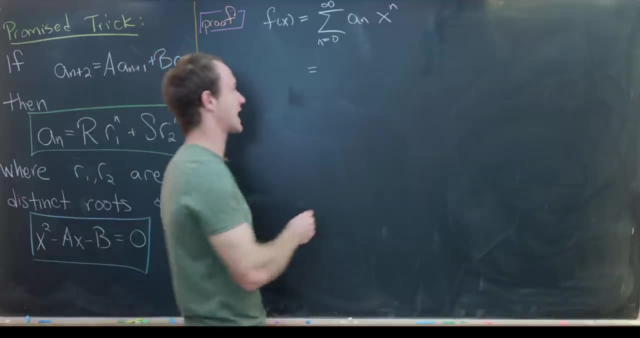 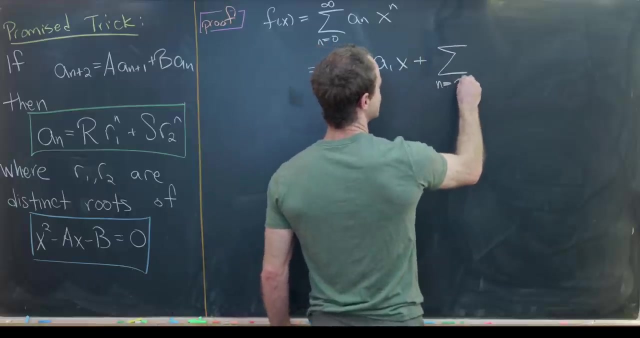 function for our recursively defined sequence. Okay, now we'll take out the first term and the second term, or maybe the zeroth term in the first term, depending on how you're counting. So we'll have a 0 plus a 1 x plus Now left over. we'll have the sum as n goes from 2 up to infinity. 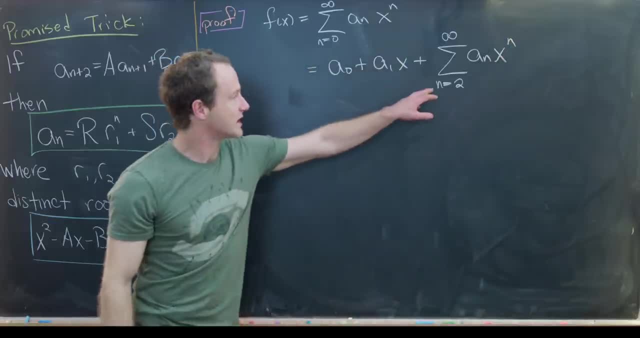 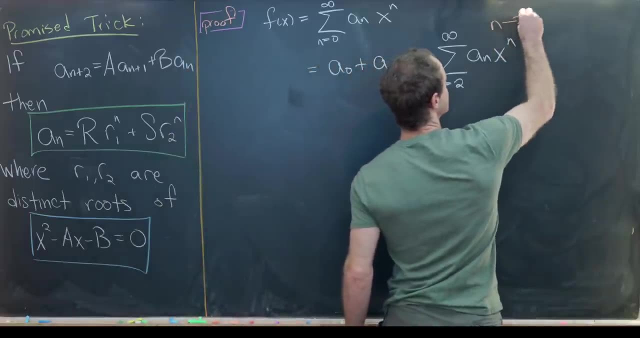 of a sub n x to the n. Now we're going to take out the first term and the second term and the second term and the second term. we can re-index this stuff right here, so that the n's are replaced with n plus 2's, and that'll be. 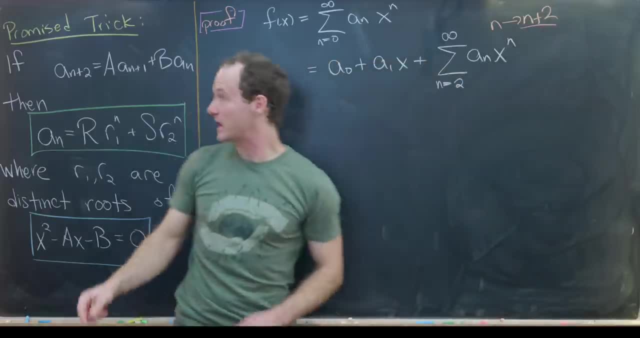 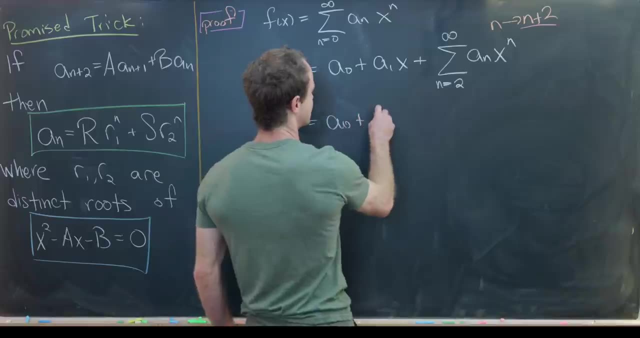 nice, because then we'll have a sub n plus 2 and we can apply our defining recursion relation. Okay, so let's see what we get. We'll have a 0 plus a 1 x, plus the sum Now n will go from 0 up to. 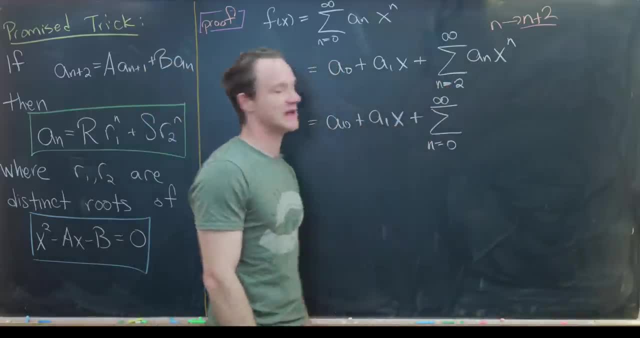 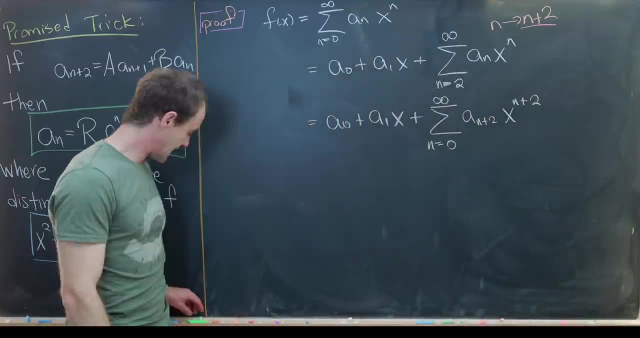 infinity, because if n plus 2 is equal to 2, n is equal to 0, and then we'll have a sub n plus 2, x to the n plus 2.. Now, next up, like I alluded to, we will apply our recursion, So I'll replace this a: 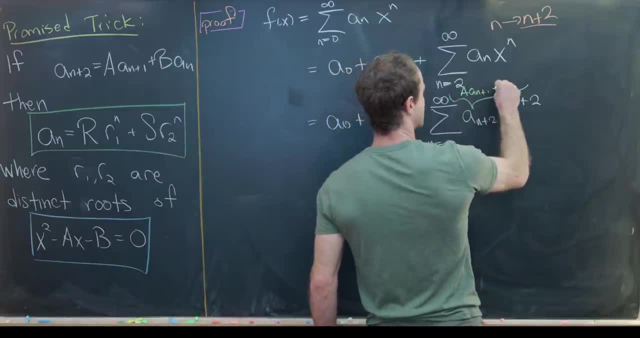 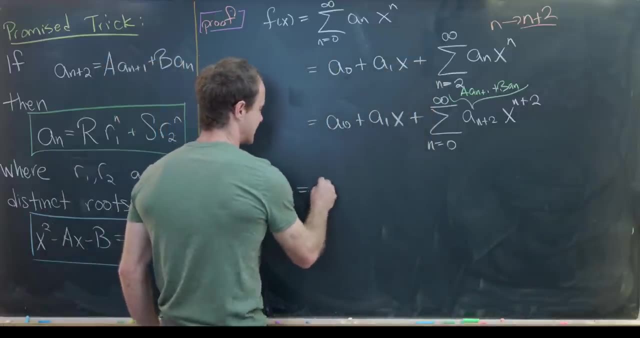 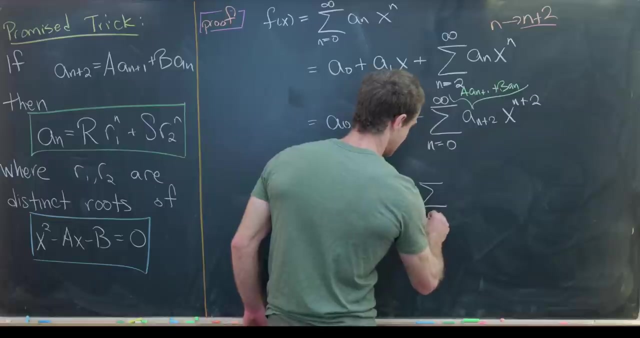 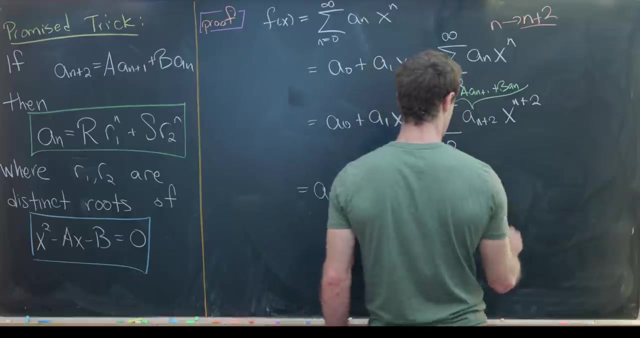 n plus 2, with capital A, a n plus 1 plus capital B a n, and then I'll pull that apart into two sums. So that's going to give us a 0 plus a 1 x plus a x times the sum, as n goes from 0 up to infinity, of a n plus 1 x to the n plus 1 plus. 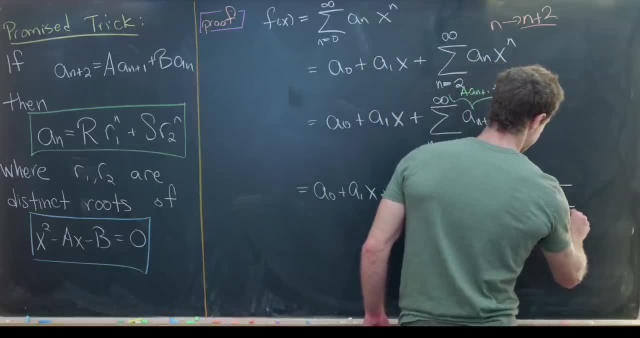 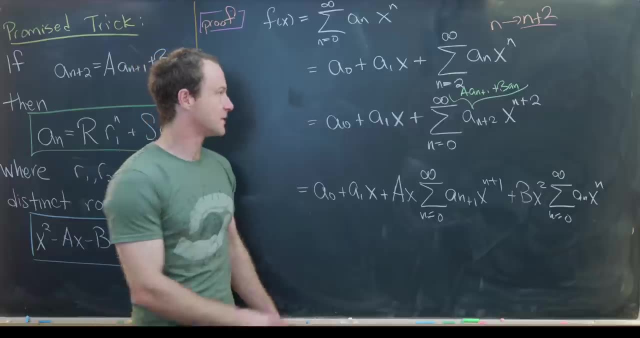 B, x squared, and then the sum as n goes from 0 up to infinity, of a n, x to the n. So I did a little bit of a simplification in the middle there. Notice, here I have a times a n plus 1 times x. 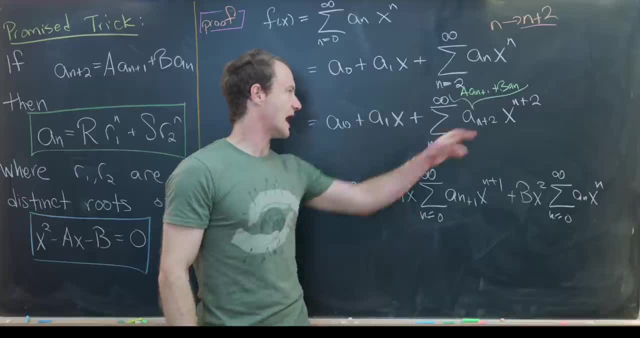 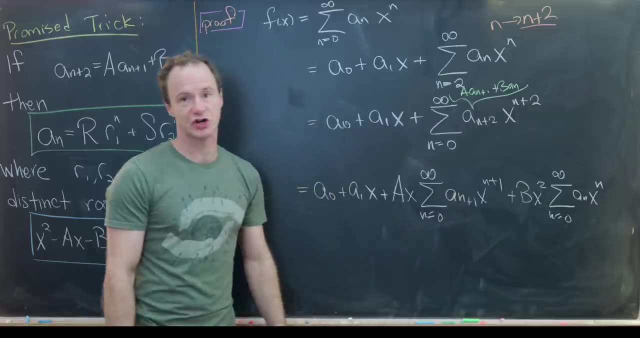 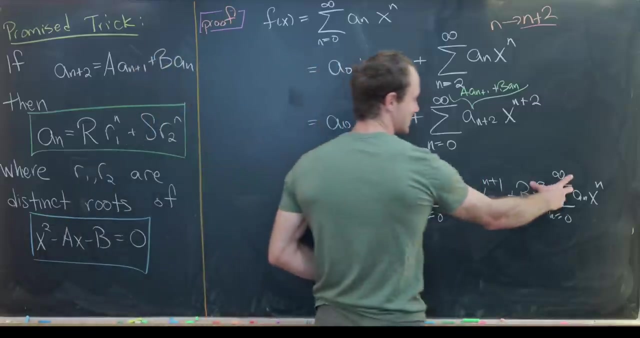 to the n plus 2.. I took our capital A And one of the x's out, leaving us with x to the n plus 1 and then the n plus first term of our sequence. We really want this index here to match with this exponent. Then I did something similar. 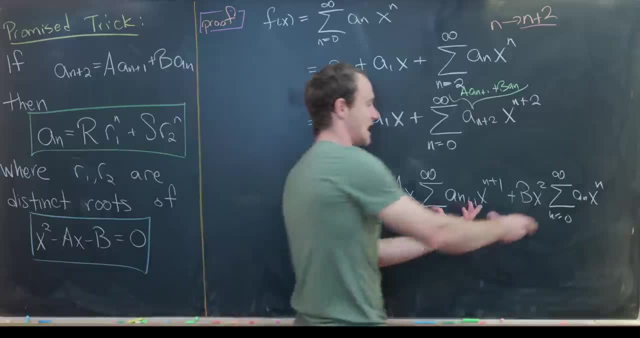 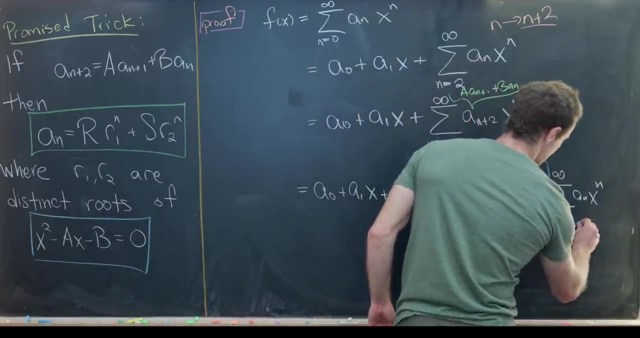 over here, But now we can notice that these objects that we've just created look a lot like our starting generating function. In fact, this one that I am squaring in blue is exactly our starting generating function, So I'm going to take this one, and I'm going to take this one, and 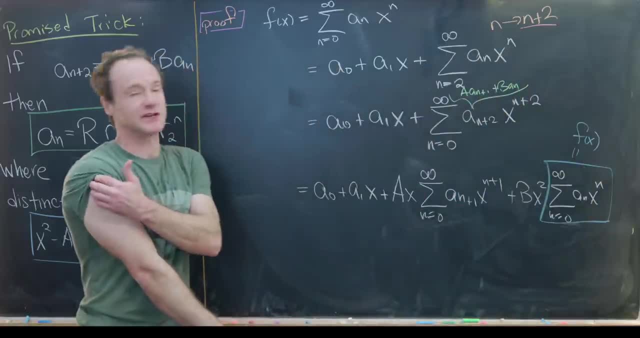 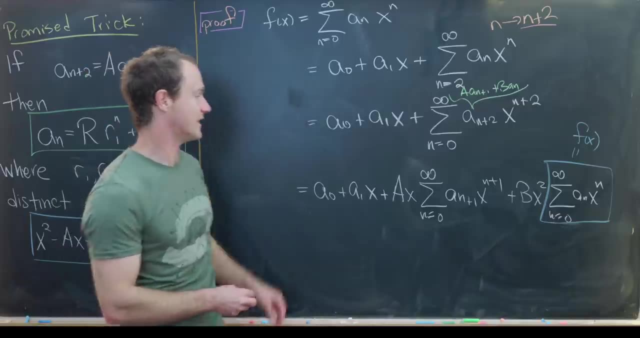 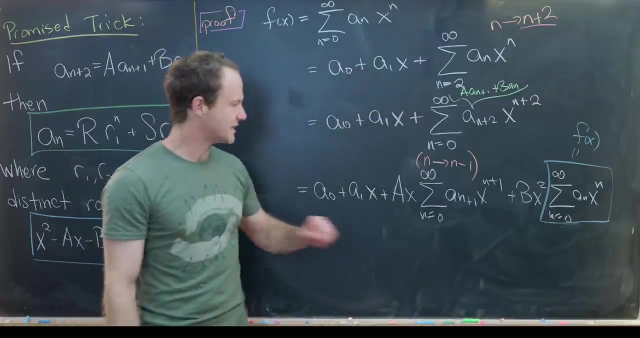 this one is almost our starting generating function. Maybe we could re-index this and see exactly how it differs from f of x. So let's maybe take n and replace it with n minus 1.. So we'll do that. So we'll have a n x to the n, and then notice: we will start at n equals 1 now. 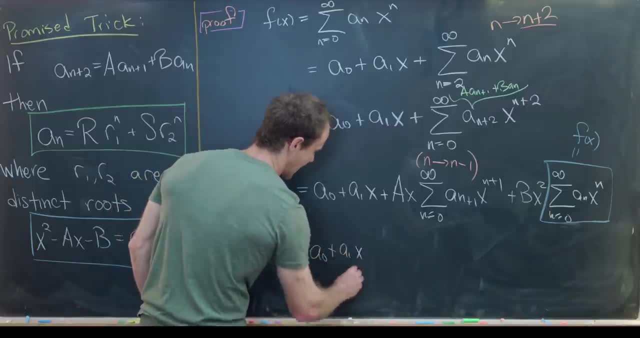 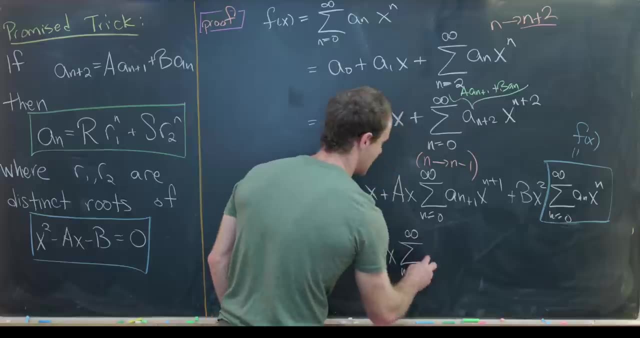 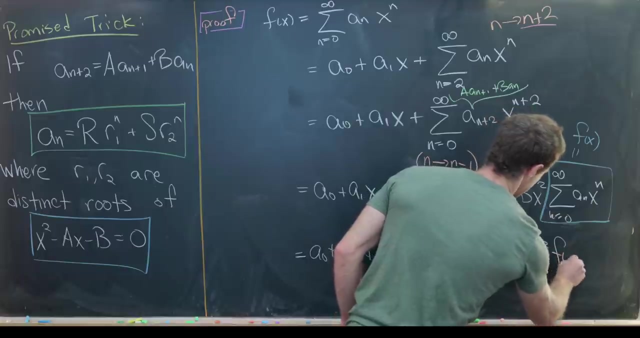 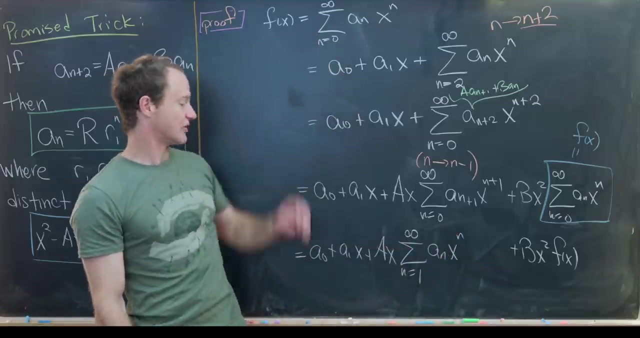 Okay, so let's write this down: We have a naught plus a, 1 x plus a times x, times the sum, as n goes from 1 up to infinity, of a, n, x to the n, And then we have plus b x squared times f of x, Like that. Now this guy right here is our original generating function. 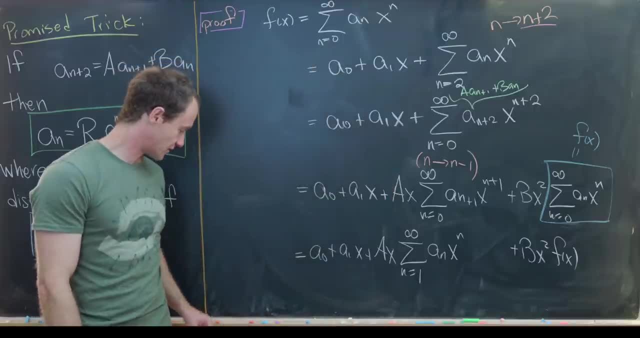 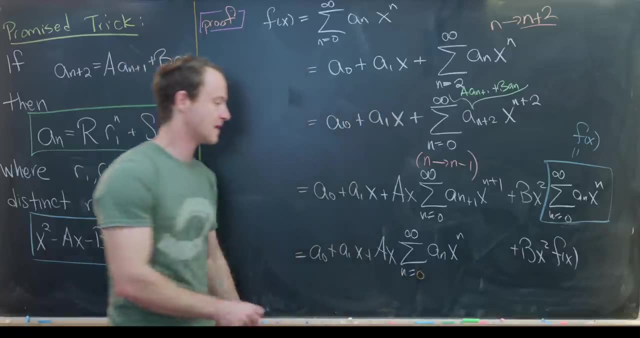 but it's missing. the n equals 0 term, But we can easily fix that. Let's add in the 0th term here. But if we add in the 0th term here, we can easily fix that. So let's add in the 0th term here. 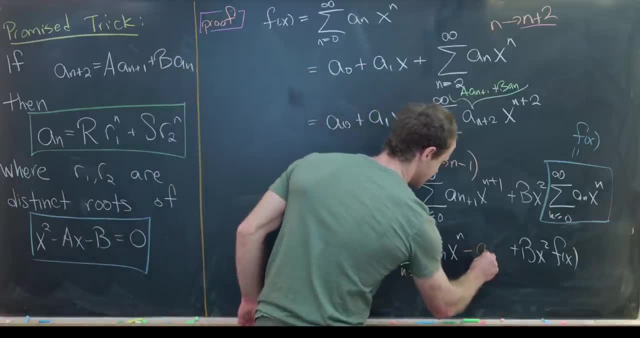 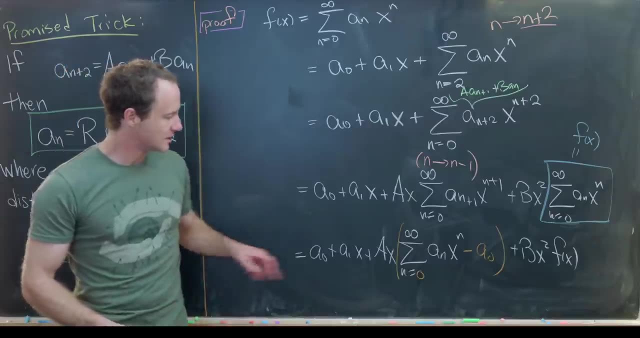 We also have to subtract the 0th term, But the 0th term is just a 0 times x to the 0, or just a 0. But let's recall that this sum was multiplied by a x. That means the correction term that we 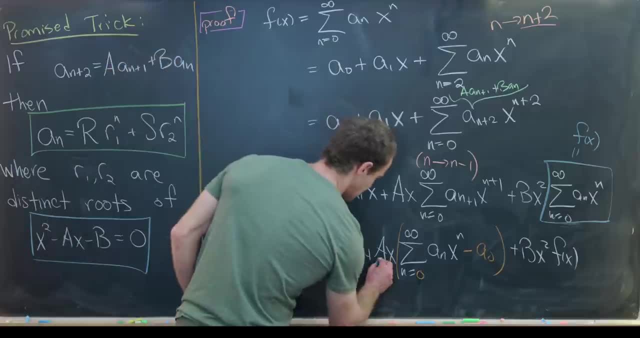 include also must be multiplied by a x. So now let's take all of this and rewrite it a little bit before we move on to the next board. So this bit right here will be equal to a times x plus a 0 times x to the 0. And then we have a 0 times x to the 0. And then we have a 0 times x. 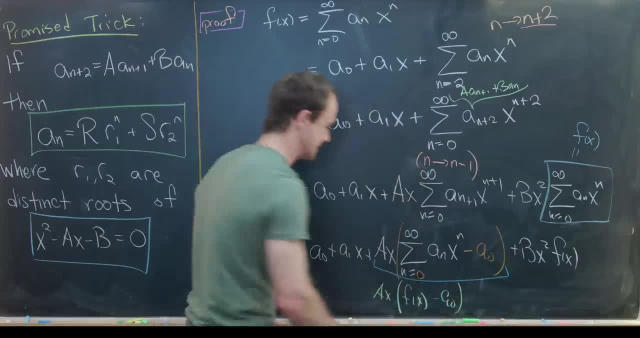 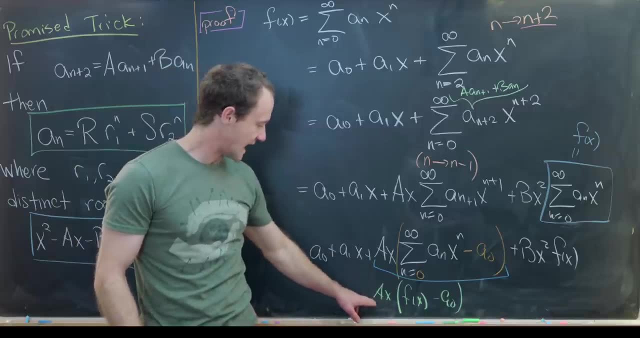 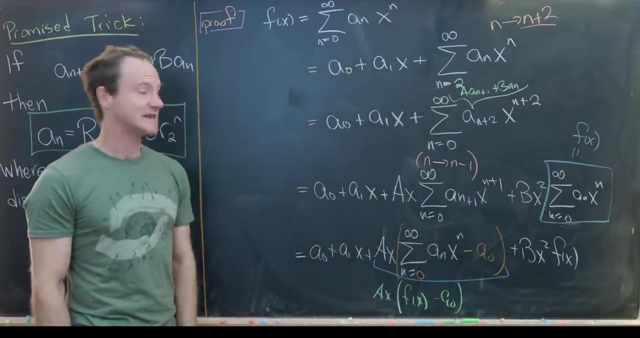 times f of x minus a 0.. So now look up here We've got f of x equals a naught plus a 1, x plus a times x, times f of x minus a 0 plus b x squared f of x. So that's a nice equation that. 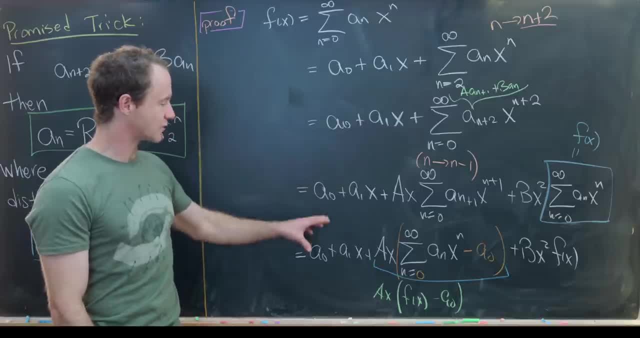 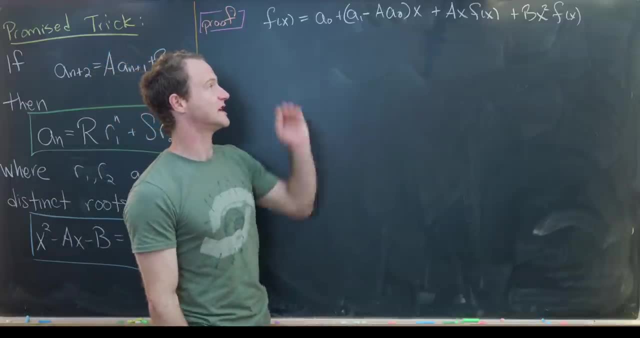 we can use to solve for f of x. But let's maybe bring the results of this board to the top and we'll move on to the next. The last calculation we did gave us the following equation: that we can solve for f of x to the 0. And then we have a 0 times x to the 0. And then we have a 0 times. 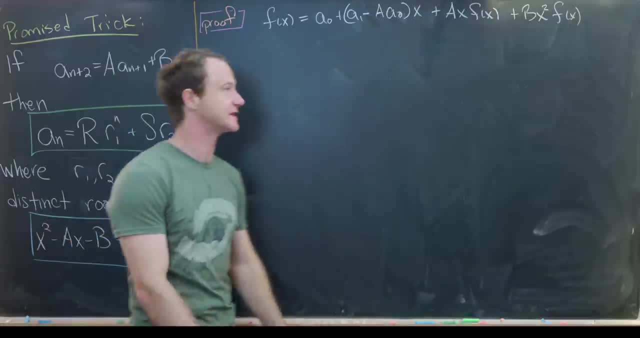 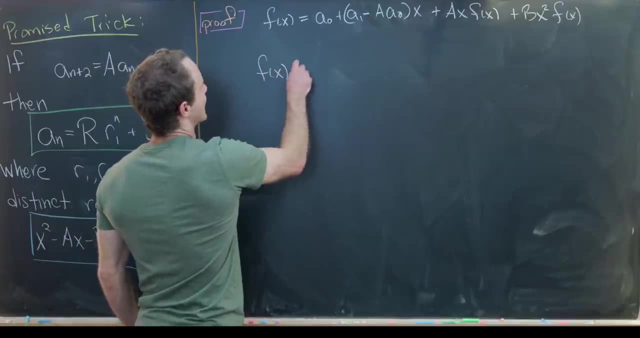 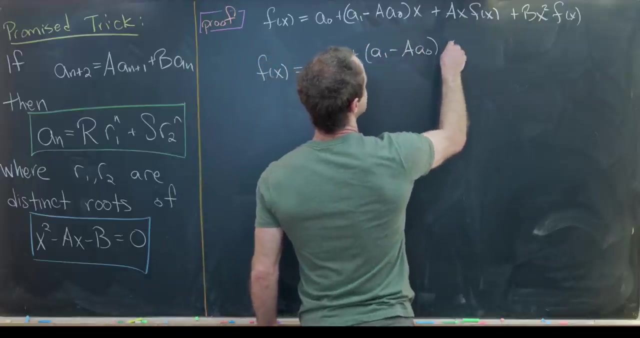 x to the 0. And then we have a 0 times x times f of x, which recall was our generating function for our recursively defined sequence. Now we can move some things around and easily solve for f of x. So let's see We've got. f of x is equal to a naught plus a 1 minus a, a naught times x over. 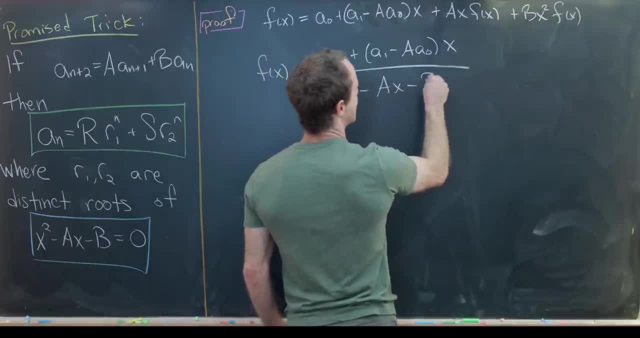 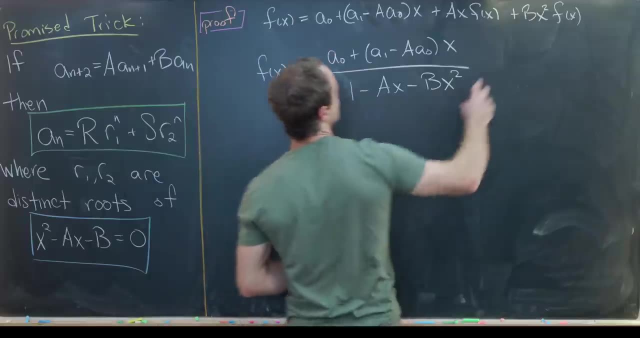 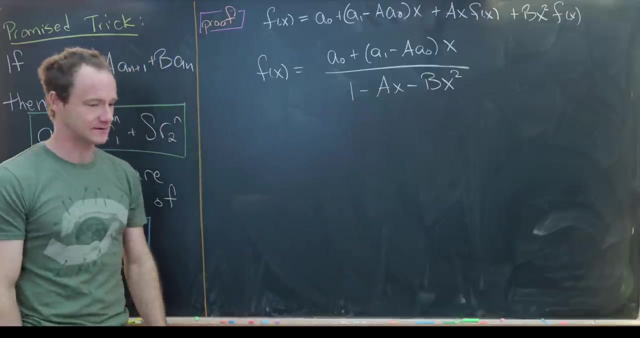 let's see, it'll be 1 minus a, x minus b, x squared. So I've combined a couple steps but we get this from moving this term over, This term over factoring an f of x out of the whole left hand side and then dividing. And now 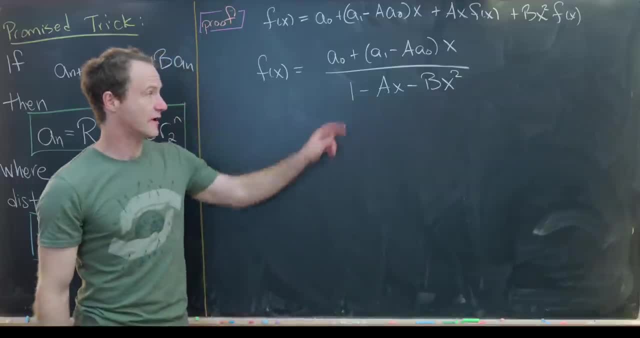 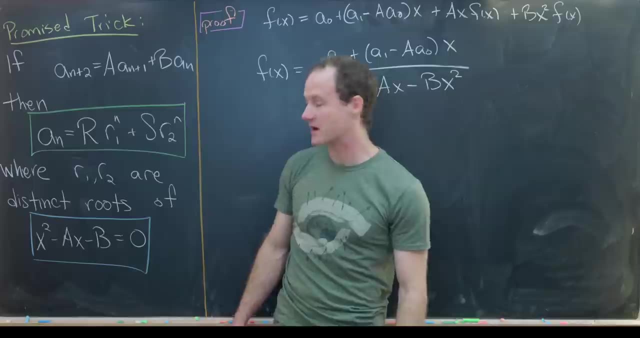 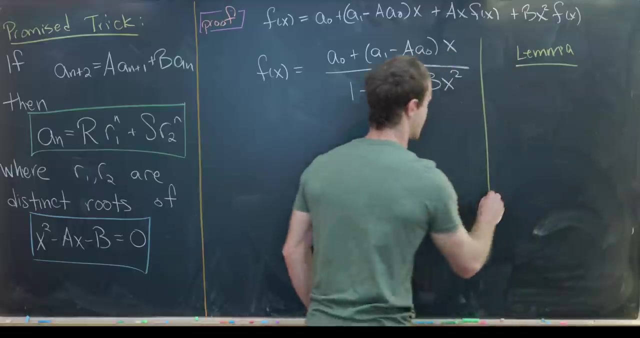 look at what we've got. We've got a linear polynomial in the numerator. We have a quadratic polynomial in the denominator, But it's not quite the quadratic polynomial that we have over here squared in blue, But it's very related to that polynomial which is over there squared in blue. 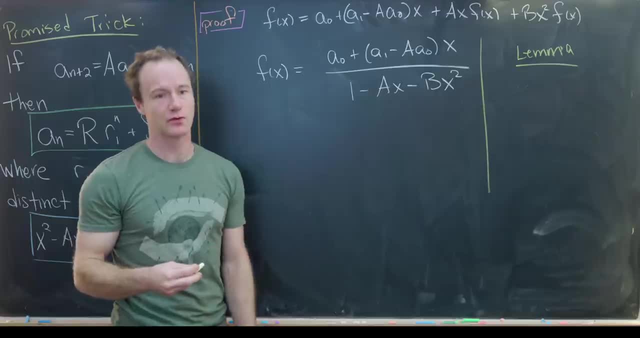 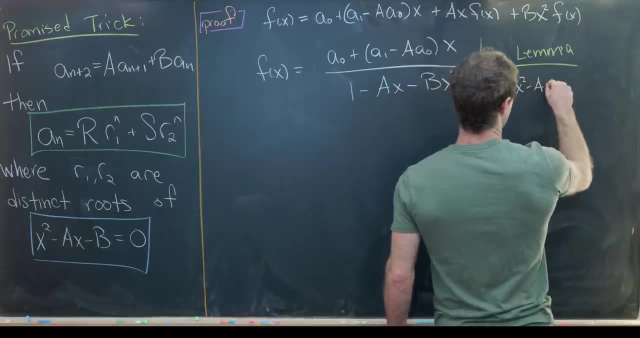 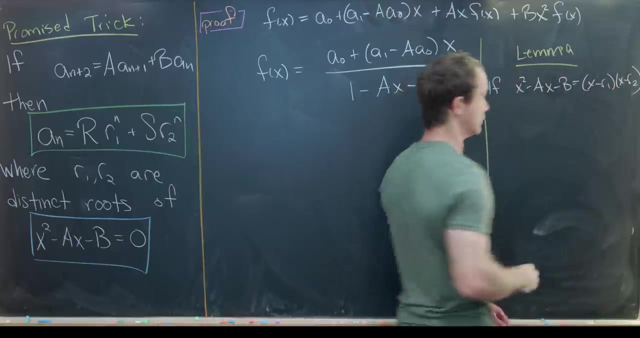 And it's related via the following lemma, which I won't prove, but I'll let you guys prove. It's pretty easy to check And that is if x squared minus a, x minus b factors as x minus r 1 times x minus r 2, which we're assuming that that happens. 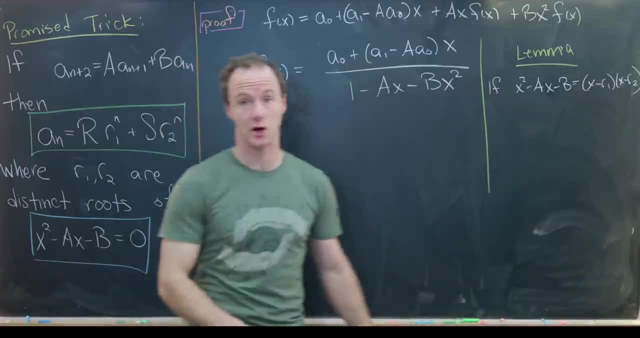 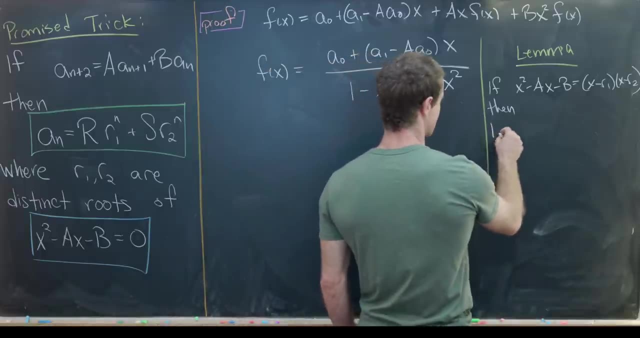 given that r 1 and r 2 are roots of this quadratic polynomial, Then the one that we have encountered factors kind of similarly. So: 1 minus a, x minus b, x squared. So we've got a: 1 minus a, x minus b. 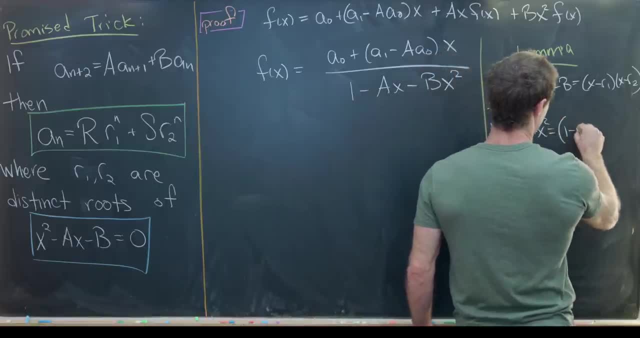 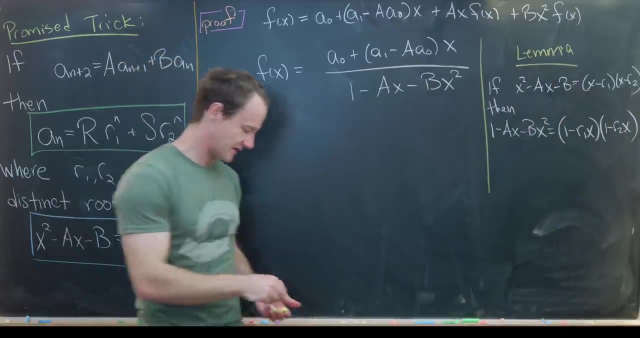 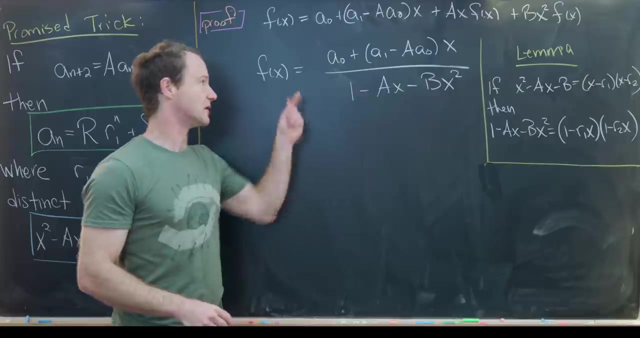 x squared Factors like 1 minus r, 1 x, 1 minus r, 2 x Great. So, like I said, I'll let you guys check that. That's not too hard to do. But now we will apply this result to our rational function version. 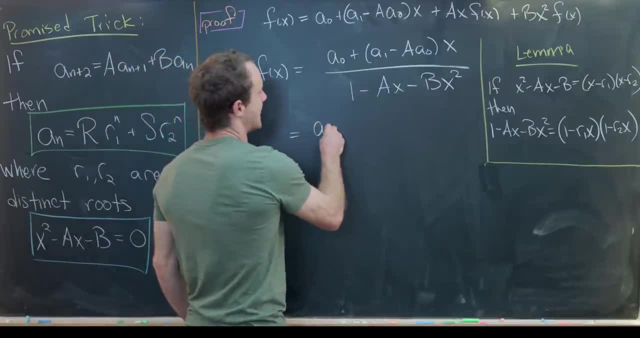 of our generating function. Okay, So let's see, We've got a naught plus a, 1 minus a, a naught x over 1 minus r, 1 x times b x squared. So that's not too hard to do. But now we will apply this: 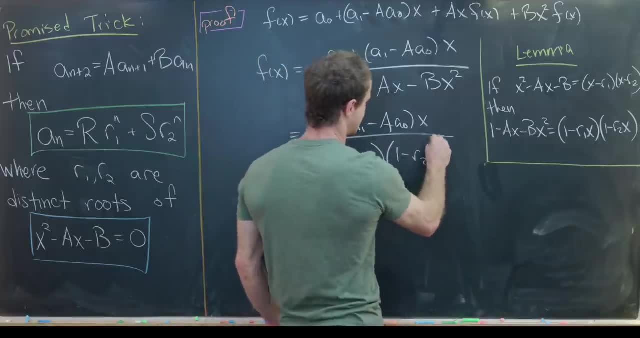 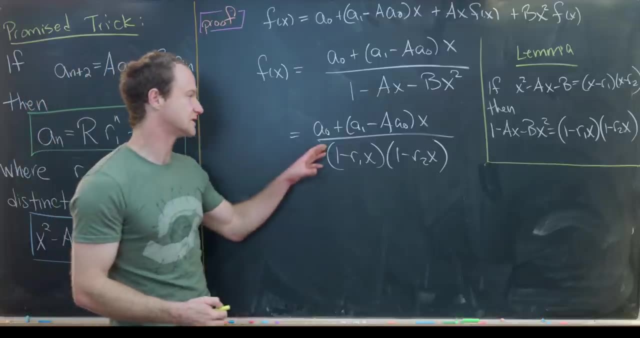 result to our rational function version of our generating function. Okay, So let's see, We've got times 1 minus r, 2 times x. But now we can do a partial fraction decomposition here, And that's possible because we have factored the denominator into distinct linear terms. So in fact this: 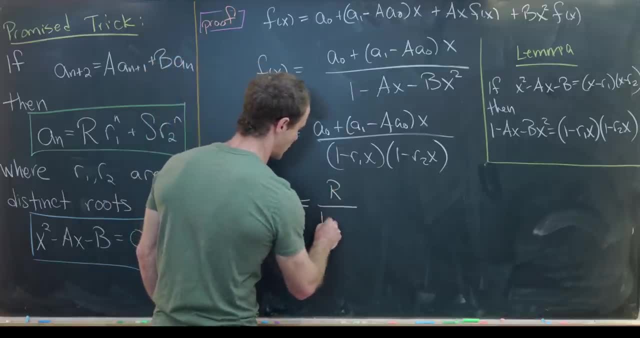 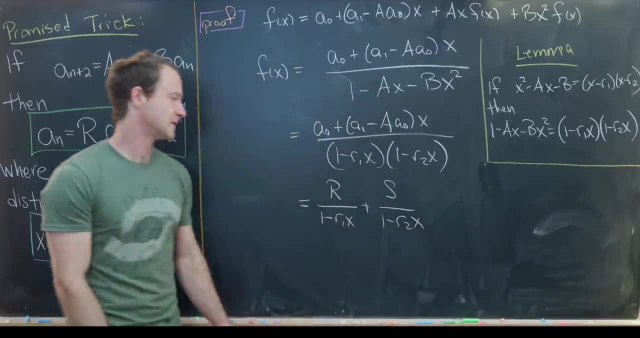 factorization will look like capital R over 1 minus r 1 x, plus capital S over 1 minus r 2 x, And here r and s. those are going to depend on the coefficient of the denominator. So we're going to do a partial fraction decomposition here. 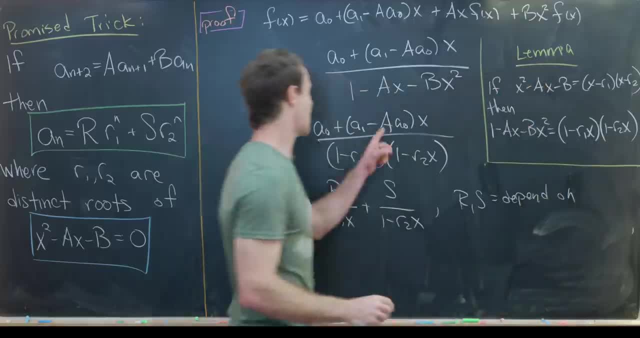 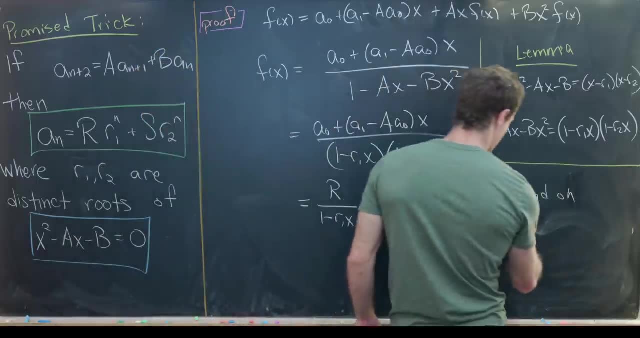 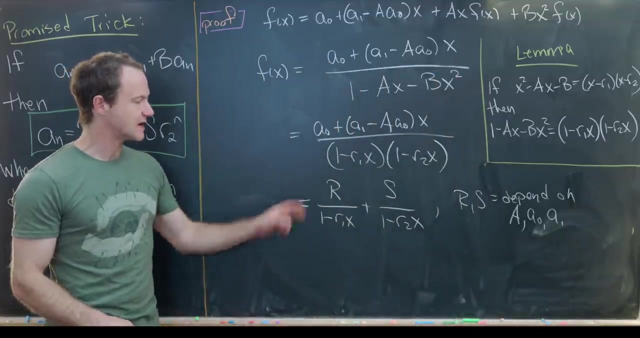 on our first term of our recursion. this capital A as well as A0 and A1. So I'll say A, A0, and A1, like that. Okay, nice, But now we can re-expand this like geometric series. 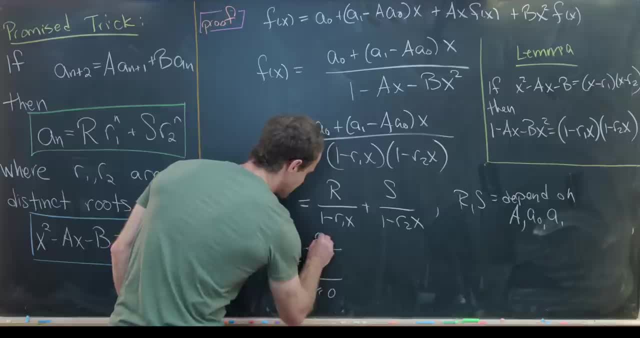 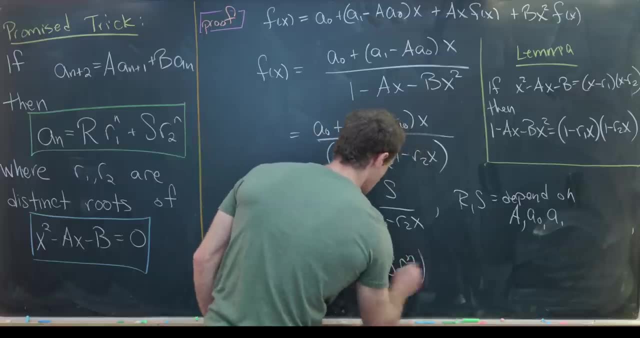 and that'll give us our sum, as n goes from 0 to infinity, of r times r1 to the n, plus s times r2 to the n, all times x to the n. So really I expanded those as two geometric series and then 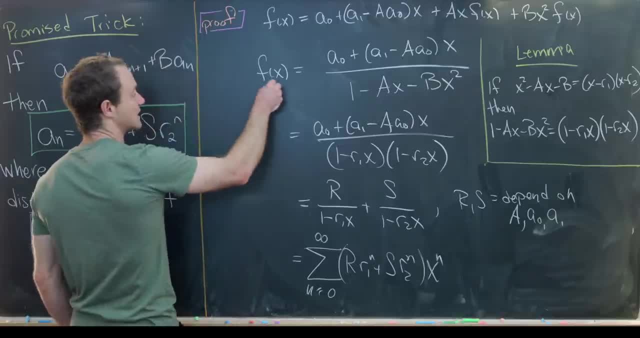 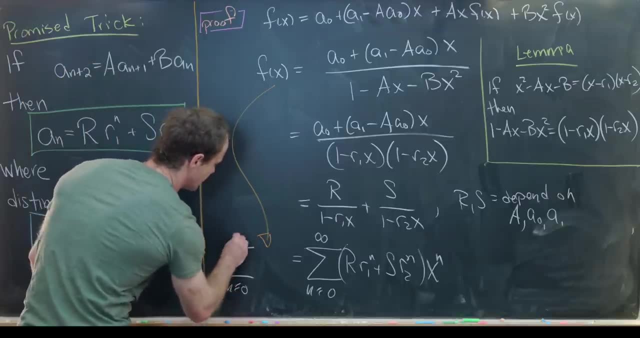 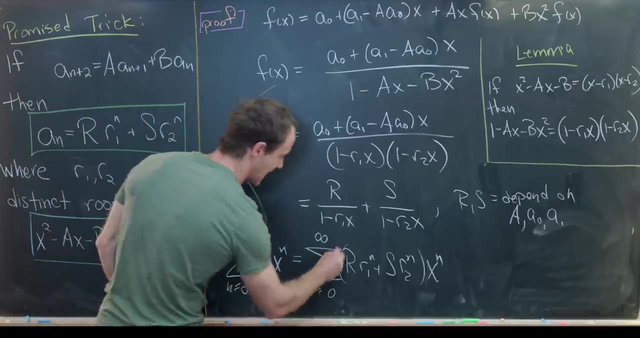 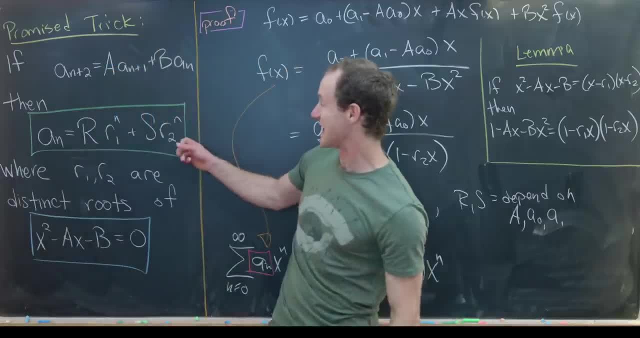 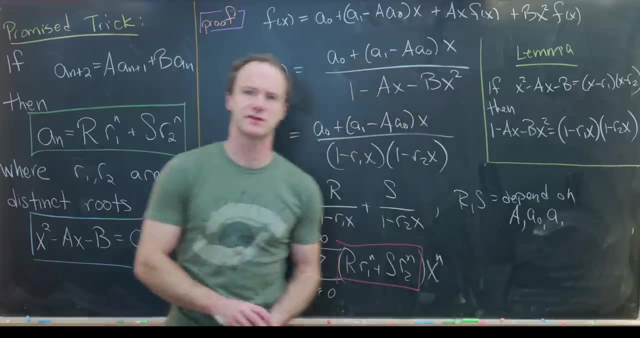 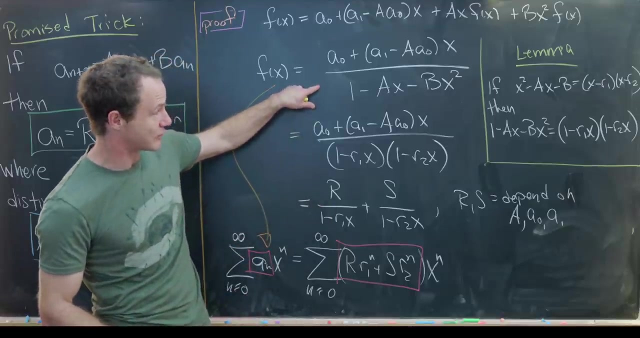 of our recursively defined sequence, And it is exactly what we would like it to be. But all of this only works if r1 and r2 are distinct roots. So what happens if they are not distinct roots? Well, luckily, we can start from this step right here with a slightly different 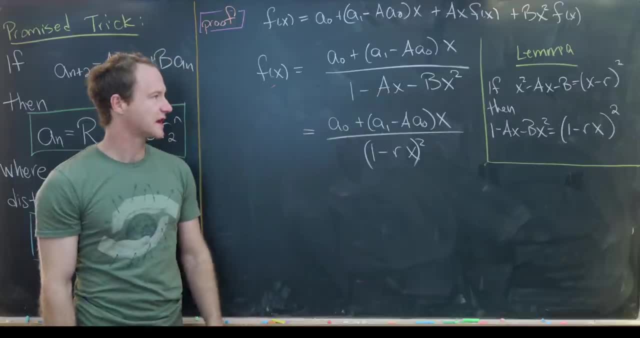 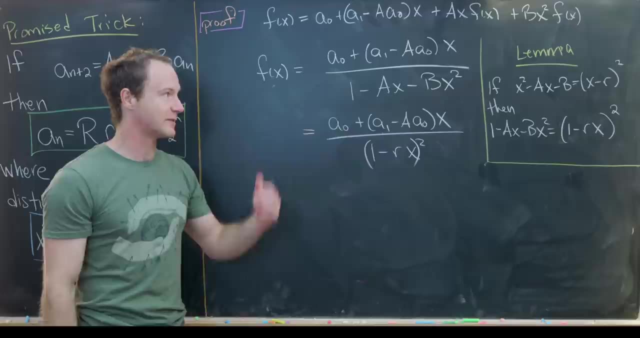 lemma and finish that off pretty quickly. So we're done looking at the case when we have distinct roots for the characteristic polynomial of our recursively defined sequence. Now we want to see what happens when we have repeated roots. So in other words, r1 and r2 are 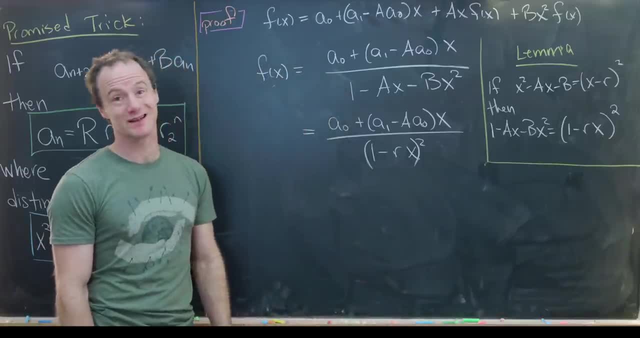 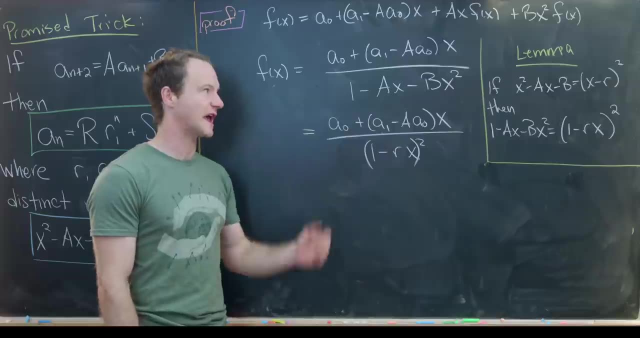 equal, and they're equal to something which we will denote by little r or lowercase r. So the following lemma follows from the lemma that we had on the last board, just for the case when you have non-distinct roots, And that is if x squared minus ax minus b. 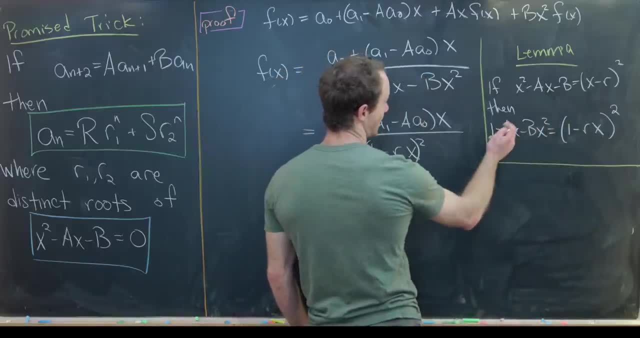 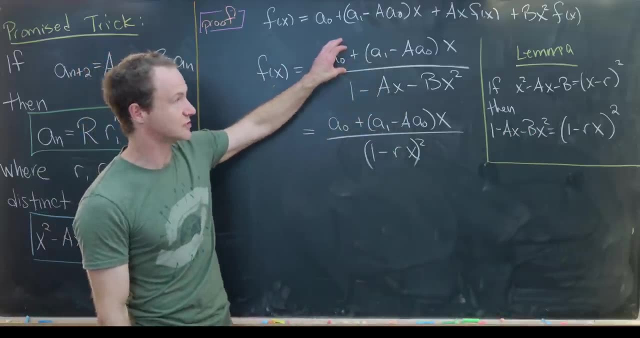 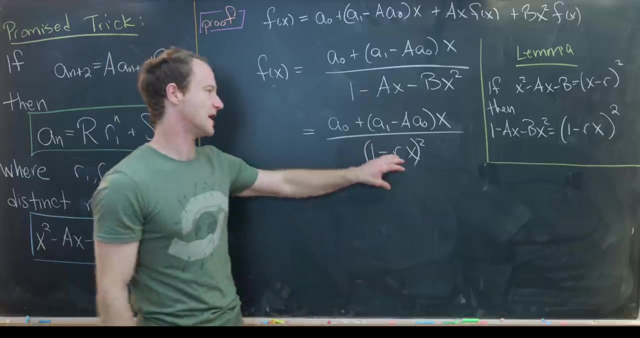 factors like x minus r squared, then 1 minus ax minus bx, squared factors as 1 minus rx. That means we can take the rational function version of our generating function and write it like this. So we've got a linear polynomial in the numerator and then this: 1 minus r times x. 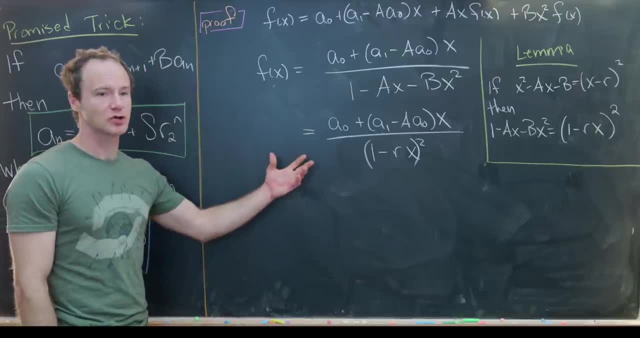 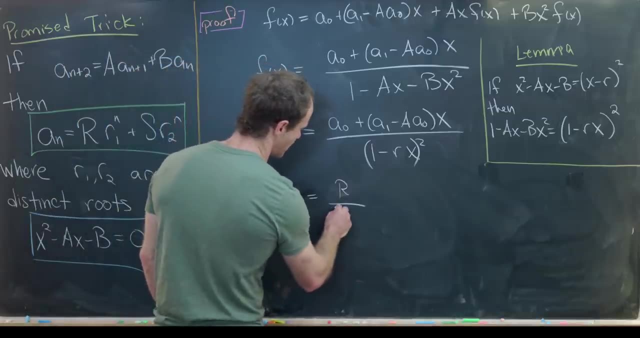 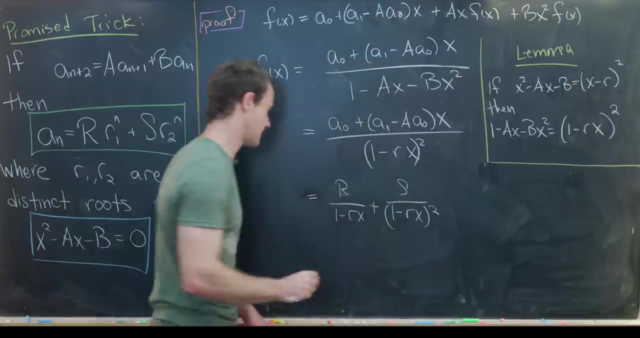 quantity squared in the denominator. But again, via some partial fraction decomposition we can pull this apart into two pieces, And now the pieces will be r over 1 minus rx plus s over 1 minus rx squared. So let's notice that if we were to put these back together we would multiply this capital. 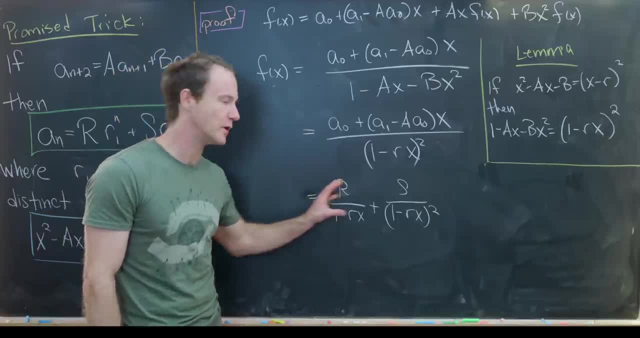 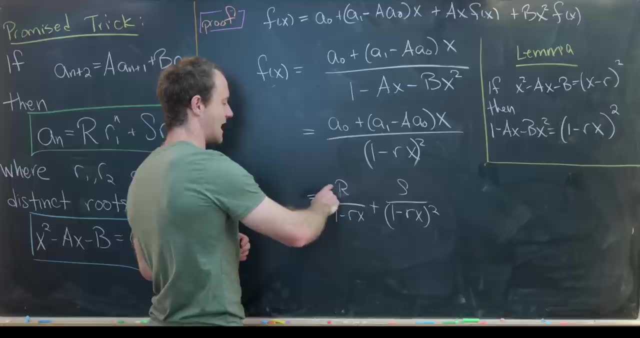 r by 1 minus rx, It would become a linear polynomial. We would add them back together and we would have a linear polynomial in the numerator. So that gives you some idea of how this. capital r and s are related to a, not a1 and capital A. 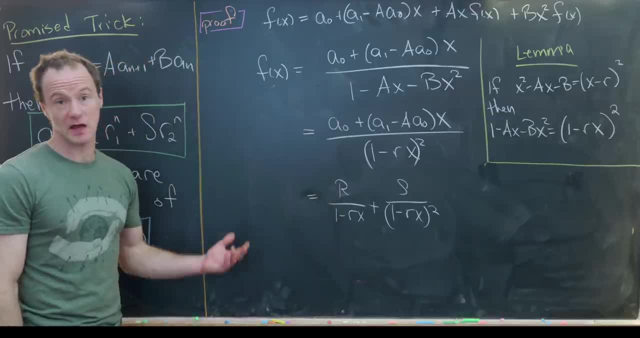 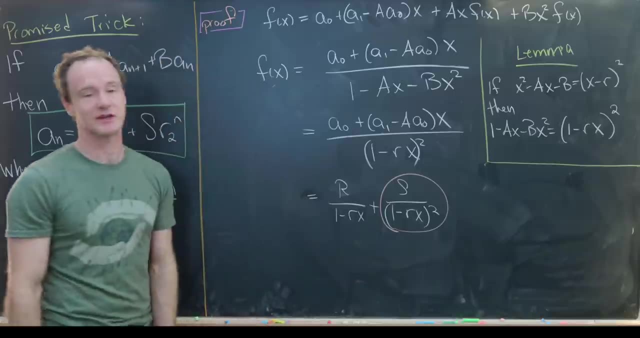 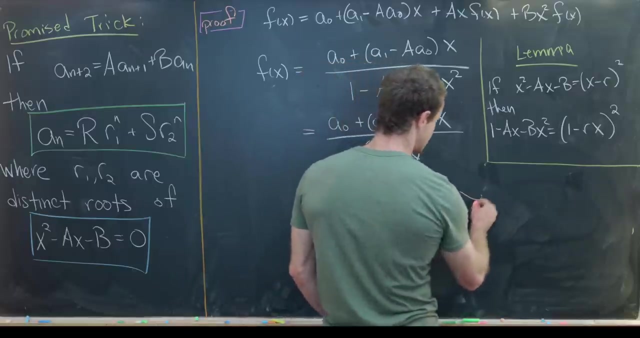 So from here we'll expand each of these kind of similar to what we did before. but we're in a little bit of trouble because this is not exactly a geometric series, But luckily it's the derivative of the geometric series. So in fact this is equal to well, let's see. 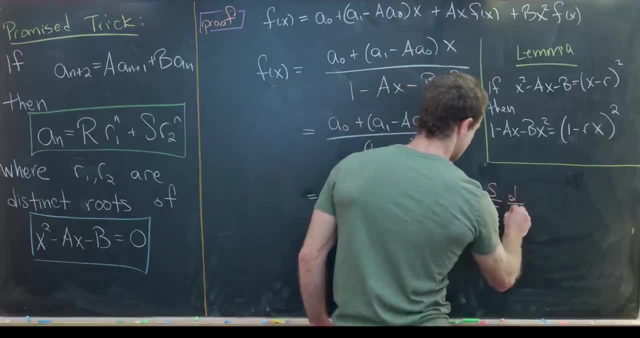 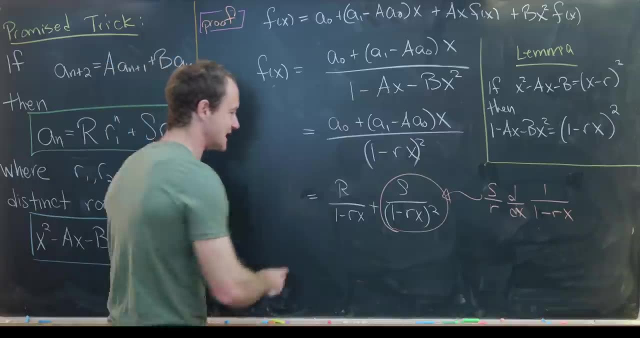 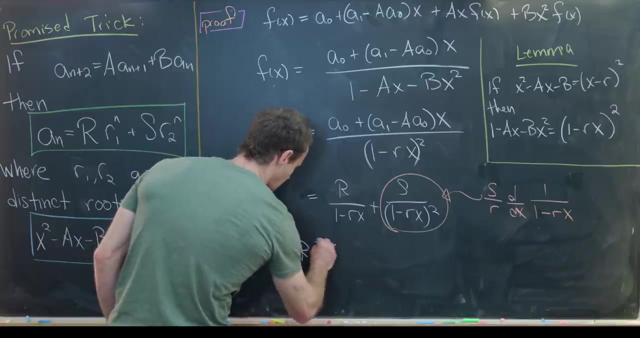 if we can get it right, s over r times the derivative with respect to x of 1 minus rx. So that means that we can take each of these, expand them, keeping in mind that we have to take the derivative of the second one. So this is going to give us r times the sum. 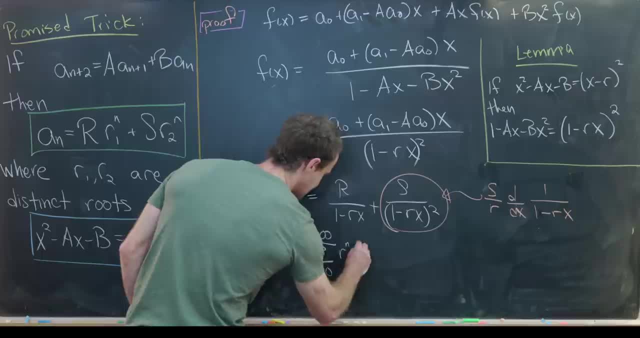 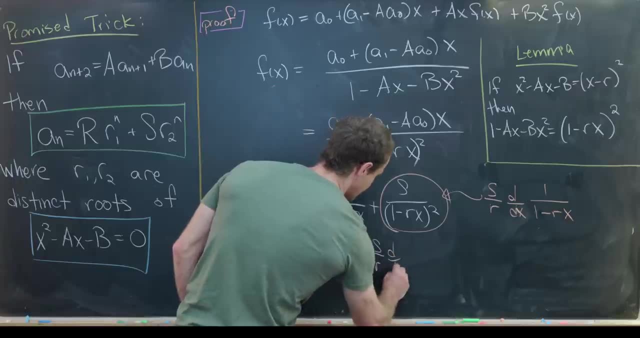 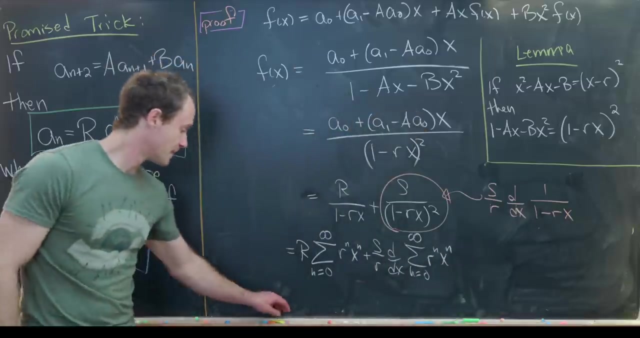 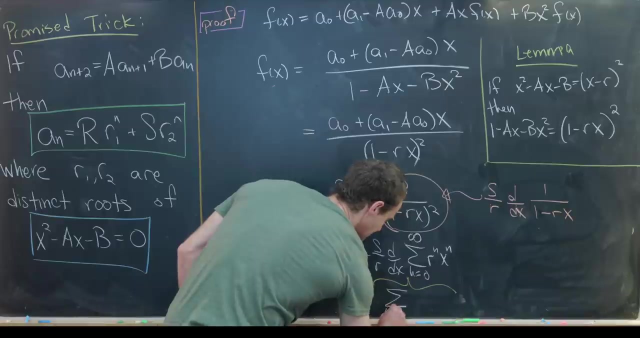 as n goes from 0 up to infinity of rn, x to the n plus s over little r. And then we'll have the derivative of the sum, as n goes from 0 to infinity of r to the n, x to the n. But that derivative is pretty easy to take, just term by term And that'll give us the sum. 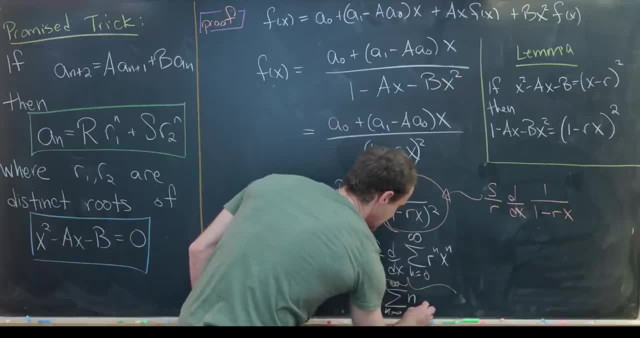 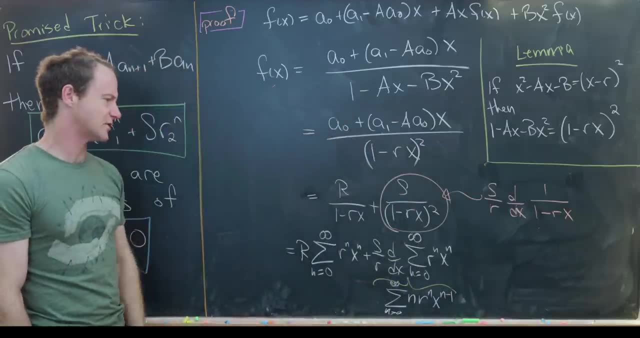 as n goes from 0 up to infinity of n times rn times x to the n. So that's going to give us the derivative of the second one. We're going to have x to the n minus 1.. Finally, we can play some tricks that are pretty similar to what we did before to push these two together. 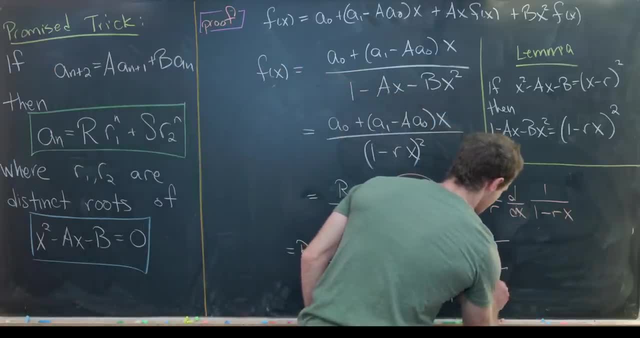 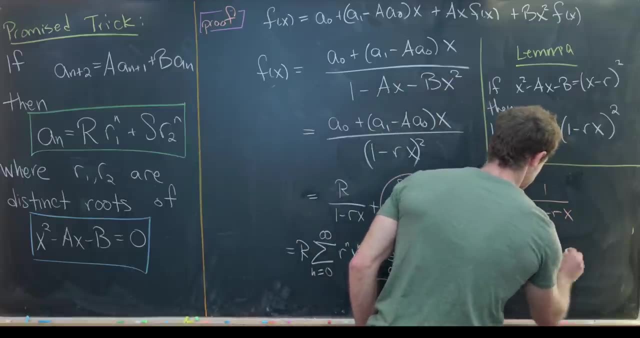 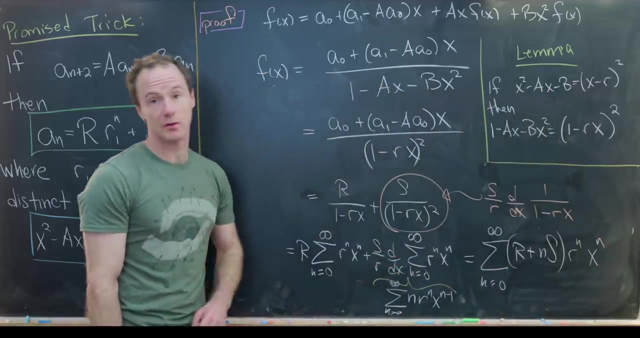 And what we will end up with is the sum, as n goes from 0 to infinity, of r plus n times s, times r to the n, x to the n Where this capital r and s have been renamed appropriately from our original r and s to. 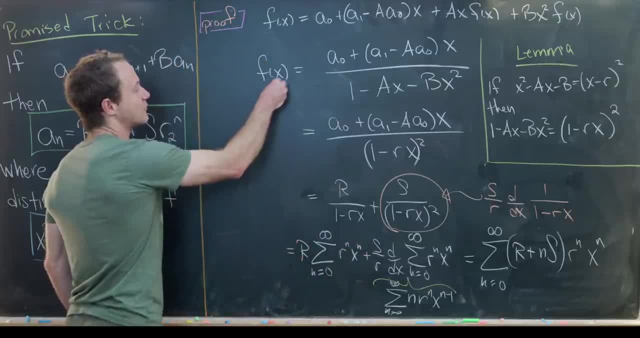 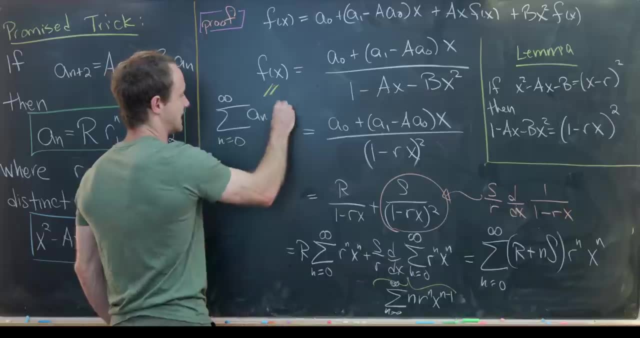 absorb any of the context constants that were there, But now rewriting f of x as its original definition, so the sum as n goes from 0 to infinity of a sub n, x to the n, and then extracting the coefficient of x to the n. 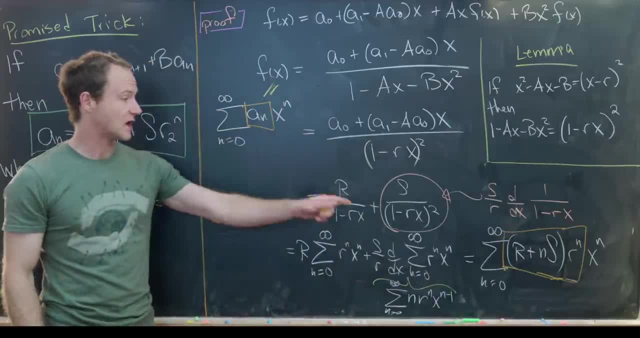 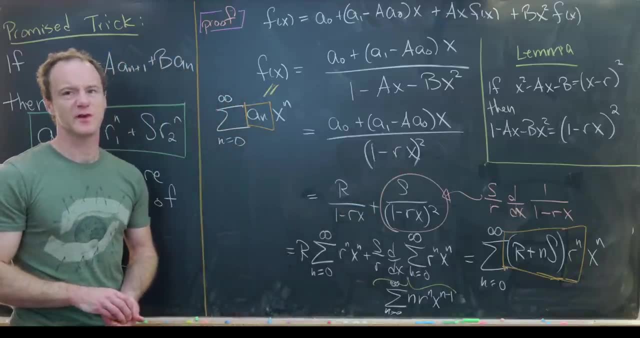 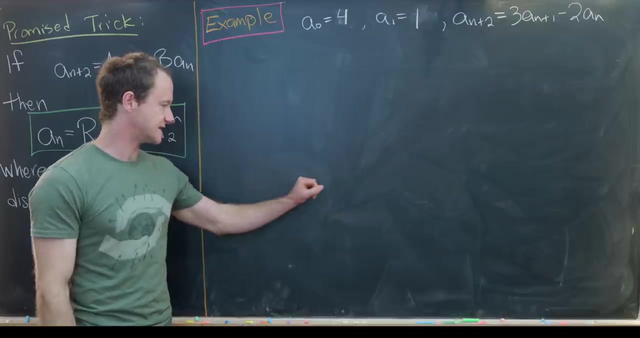 from both sides. we see that we've found a closed form, in this case, where we do not have distinct roots. Okay, so, let's finish this video off with a quick example. Okay so, let's finish this off with one example. So let's say we've got the following recursively defined sequence: So the 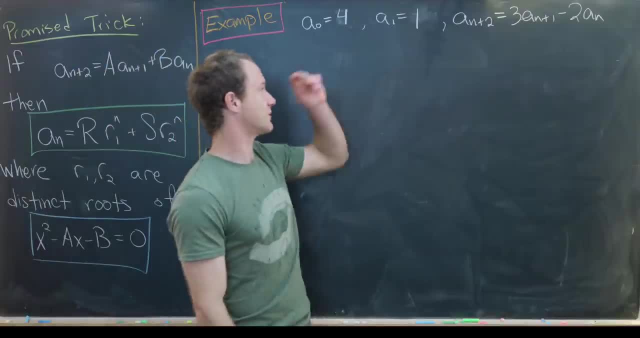 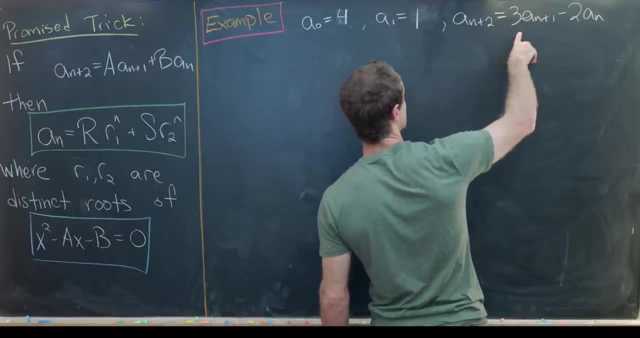 zeroth term, a0, is 4,, the first term, a1, is 1, and then our two-step recursion is given as follows: So a n plus 2 is equal to 3 a n plus 1 minus 2 a n. So what we've got over here gives us a nice. 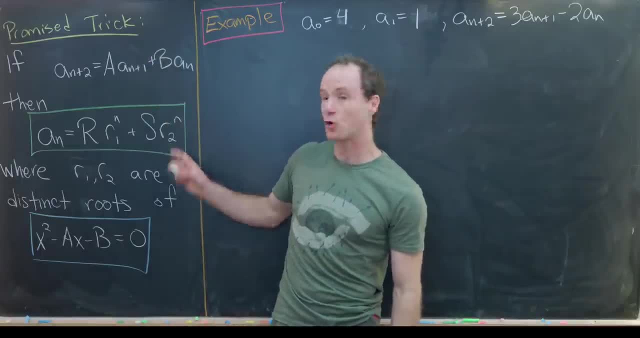 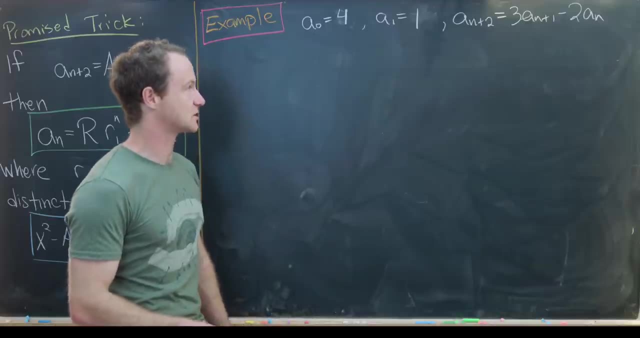 polynomial which we should look at and that'll allow us to quickly write down a rough draft of the closed form that we can maybe tweak. Okay, so let's jump into it. So we'll look at maybe this thing that I'm calling the characteristic. 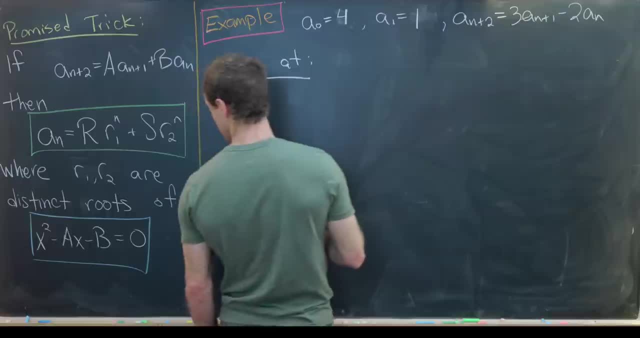 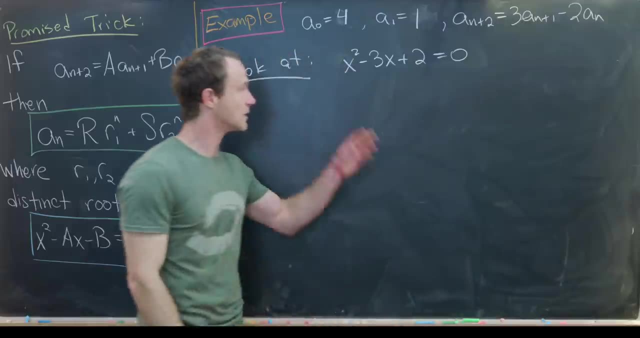 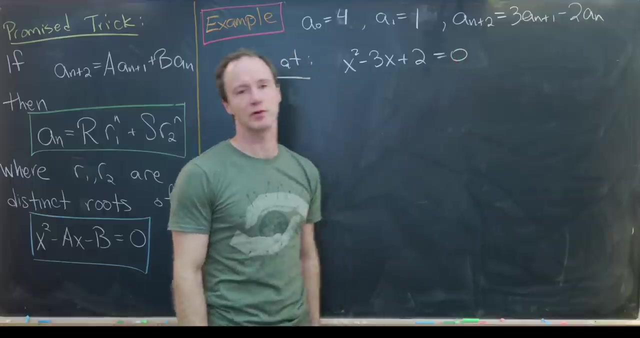 polynomial of the recursively defined sequence. So in this case it will be: x squared minus 3x plus 2 equals 0.. We need to find the roots of that. That's because capital A- here, like over here, is equal to 3 and capital B is equal to negative 2.. All right, but now let's notice that. 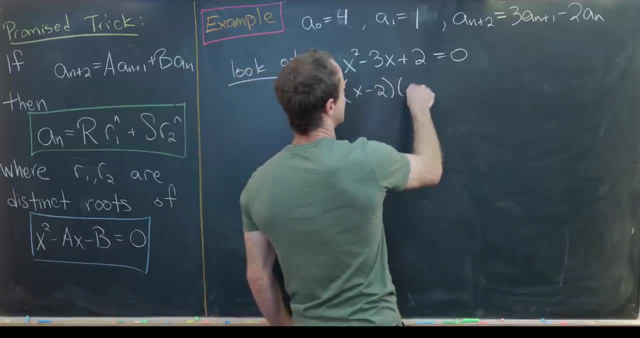 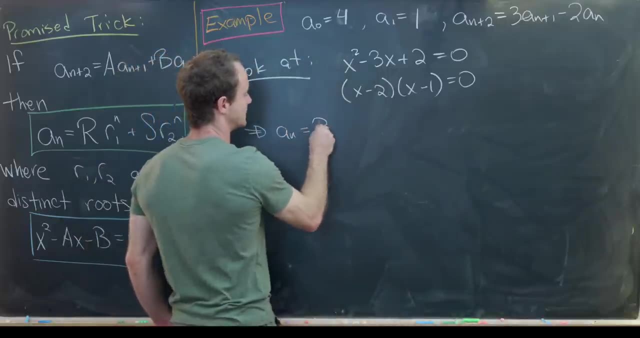 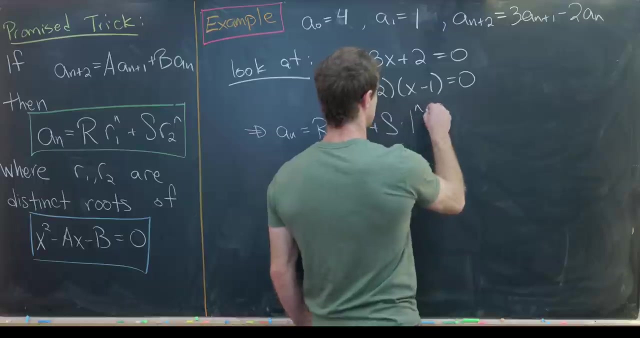 this thing factors pretty nicely. This is x minus 2 times x minus 1 equals 0.. Okay, so that means a n is equal to capital R times 2 to the n, plus capital S times 1 to the n, Because 2 and 1 are the roots. 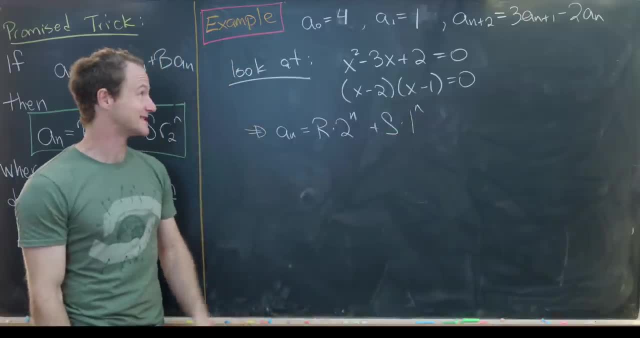 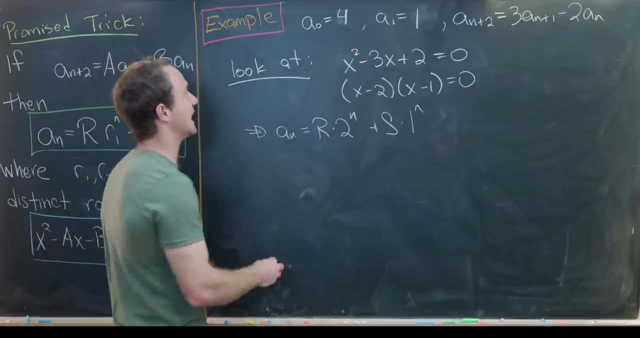 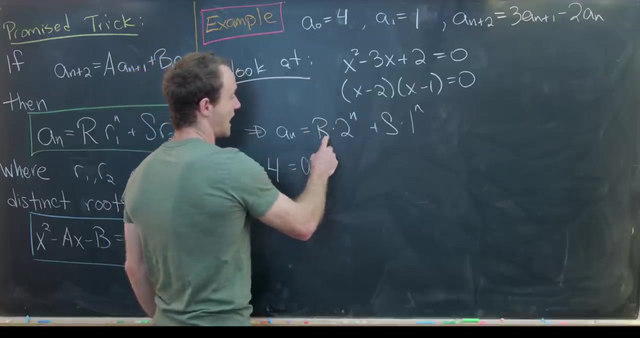 to that polynomial. Well, obviously 1 to the n is always n, so that's not super interesting. But now we can apply these initial conditions to find values of r and s. So let's notice that on the one hand we are given that a 0 is 4.. But on the other hand, 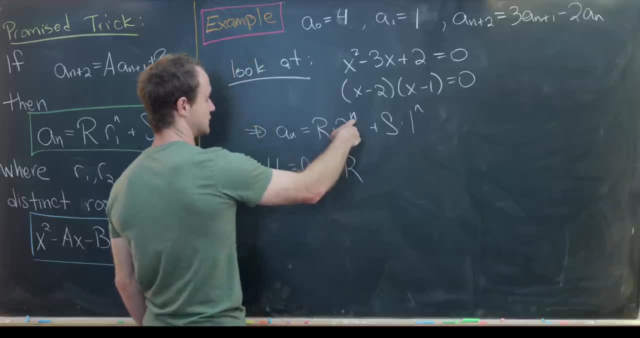 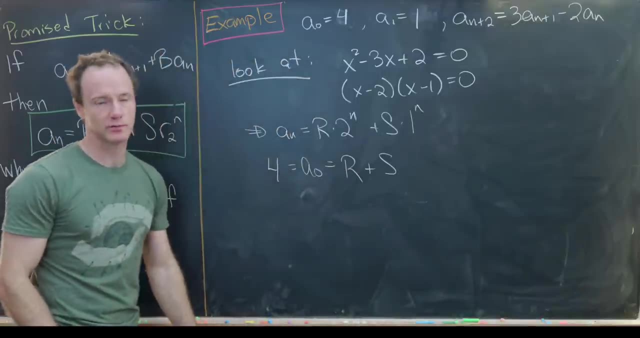 we know, a 0 has the form r times 2 to the 0,, which is 1, plus s times 1 to the 0, which is also 1.. So we've got this equation: 4 is equal to r plus s, And then, likewise, we're given that a 1 is: 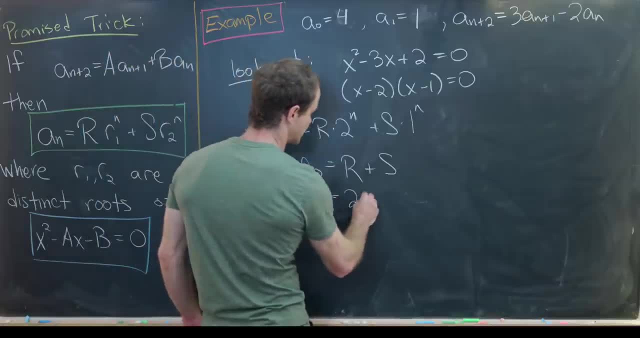 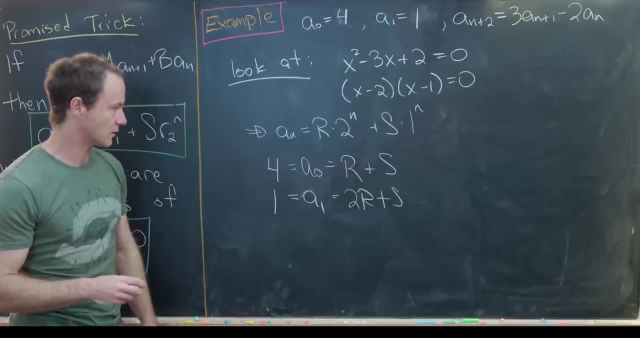 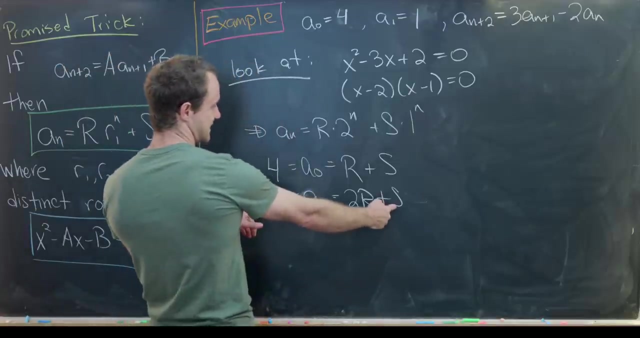 equal to 1.. But on the other hand, it's equal to 2r plus s. Just by plugging 1 into this rough draft of our closed form, That gives us a system of equations for r and s. Let's see what we can do with it. Maybe we'll take this second equation and subtract the first. 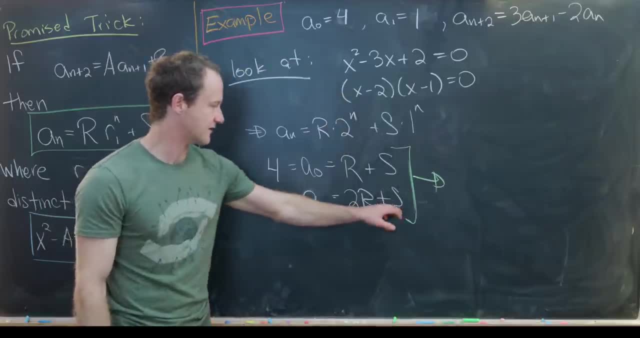 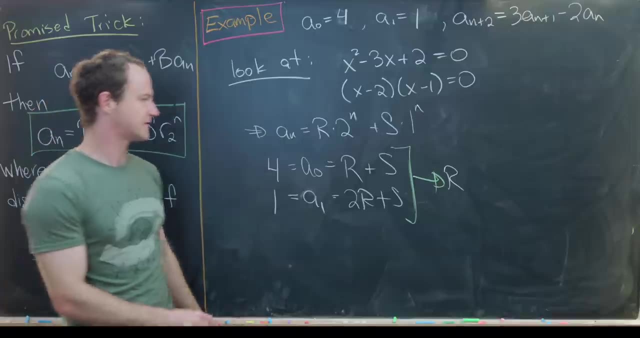 equation, So that'll have the nice simplifying effect of getting rid of the s. So we'll have: 2r minus r is just r, And then we'll have 1 minus 4 is negative 3.. So that means this number, right. 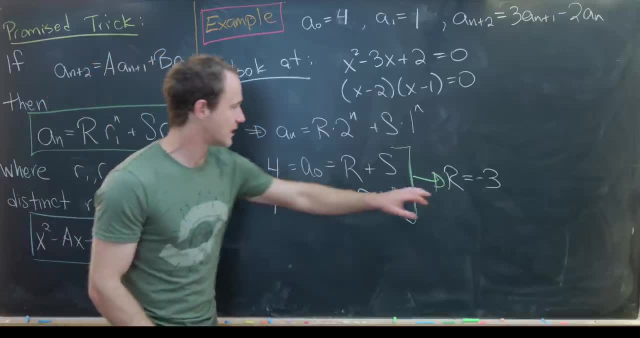 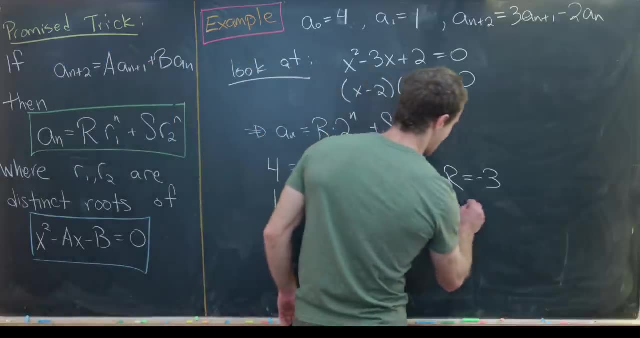 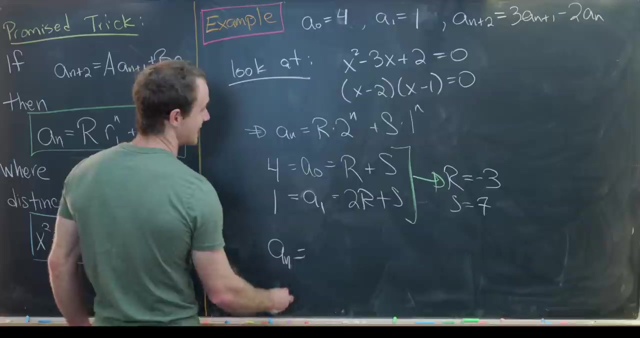 here must be equal to negative 3.. But now we can plug this value of r into either of these two equations in order to get a value for s, And you'll see that s is equal to 7.. So that finally gives us our closed form. an is equal. 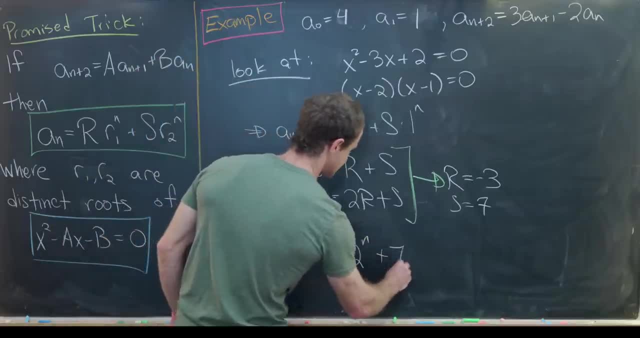 to minus 3 times 2 to the n plus 7.. And that's a good place to stop. 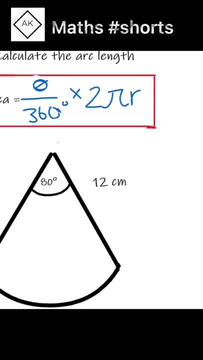 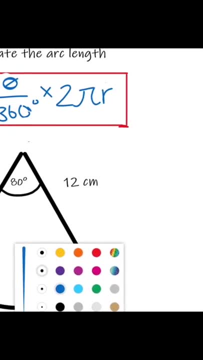 This video will show you how you can calculate the arc length of any sector. So the arc length formula is angle theta over 360 degrees multiplied by 2 pi r. So if you use the values provided in the sector diagram, we know that the angle theta in this case is 80 degrees and that the radius 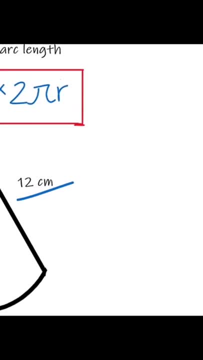 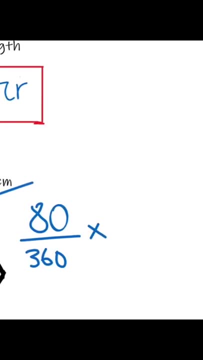 of the sector is 12 centimeters. So we use the formula, we substitute the values in so that we work out 80 degrees over 360 degrees. So we're dividing it, multiply by 2, multiply by pi, multiply by the radius, which in this case is 12 centimeters, and then we put this into our scientific calculator. 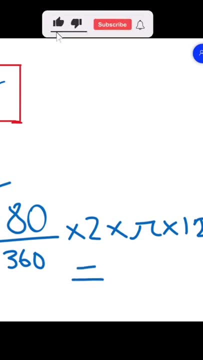 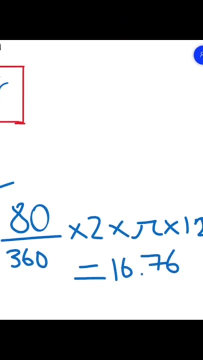 to give us an answer of 16.76 centimeters to two decimal places, and it doesn't state what decimal place it wants us to give the answer to. so you can choose an appropriate decimal place to give it to and you must state any answer. So that's how you calculate the arc length of